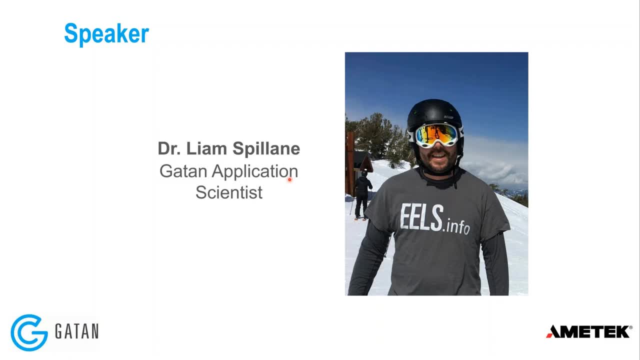 eels doing applications, the chief application scientist at Gatan, And he also has done a fair amount of programming within Gatan so he also has helping us with the GMS workforce. So he will be taking over today for the presentation. Just a bit of housekeeping, If you. 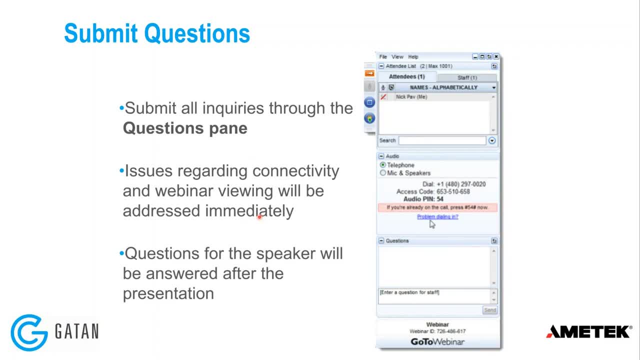 have any questions about connectivity or data or image quality, sound quality. please send that question in. We'll try to get to those right away. Questions about the content: we'll hold to the end and we'll try to get to those questions. If we can't get to them all at the end, we'll follow up. 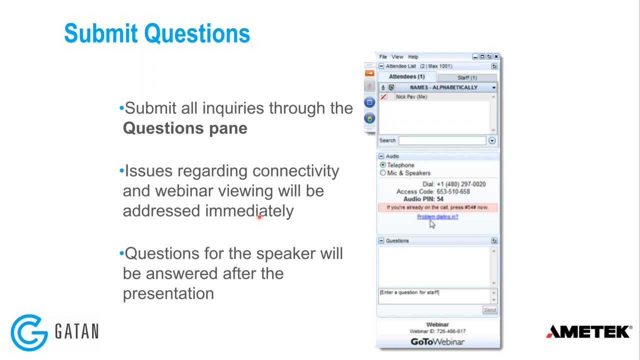 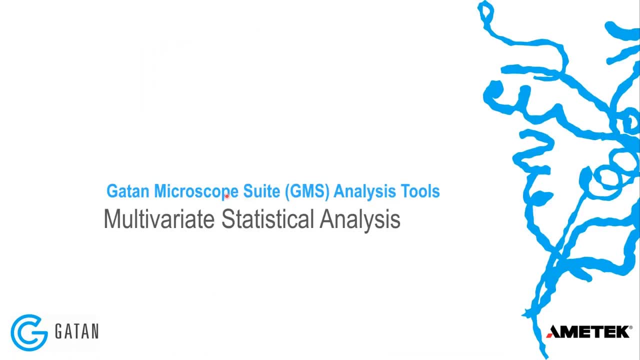 by email. We get a record of all those questions. All right, Without any further ado, I'll hand this over to Liam to take over the presentation. Thanks, Liam. Okay, Thanks very much, Ray, And thanks to everyone for tuning in. So fourth webinar in the. 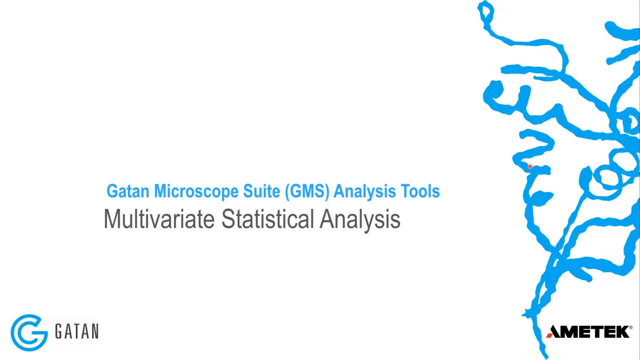 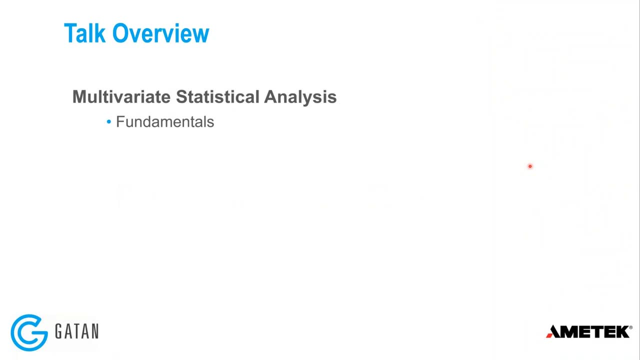 webinar series- multivariate statistical analysis. So a brief overview of the presentation. So I'm going to start off covering some multivariate statistical analysis fundamentals. Then I'll go over how we approach this in our software. So an overview of the new software tool. 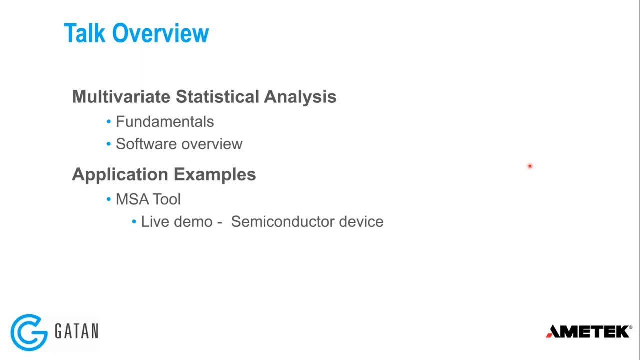 And then we'll move on to some application examples. So the first application example is going to be a live demo of the new tool. Actually, it's from a multilayer bismuth ferrite device. We might look at the semiconductor device as well, And then I'm going to show you how to use external packages, if 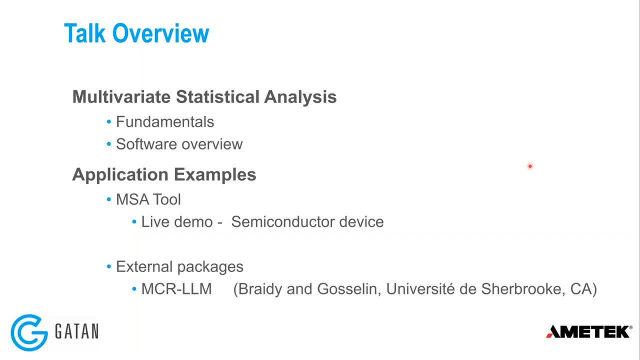 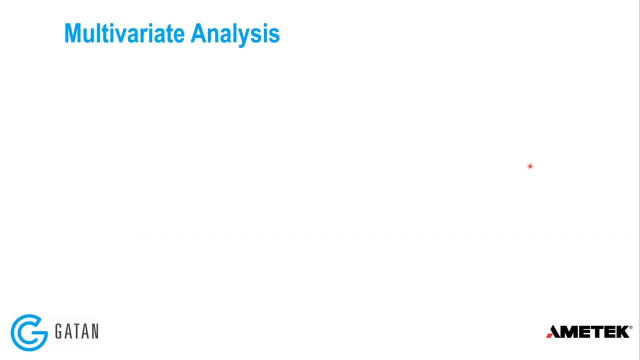 you want to use something non-standard. So the package that I'm going to be using is this MCR LLM package, which is a multivariate code that was written by Professor Brady and Goslin out of University de Sherbrooke, which is in Canada. So, multivariate analysis. what is it? The EEL spectrum? 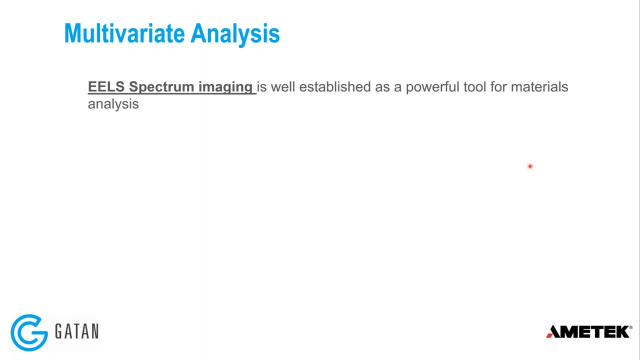 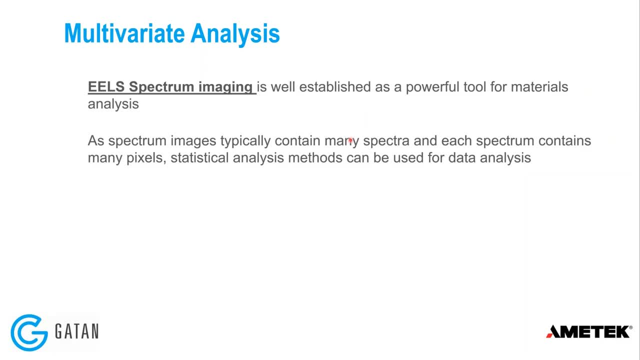 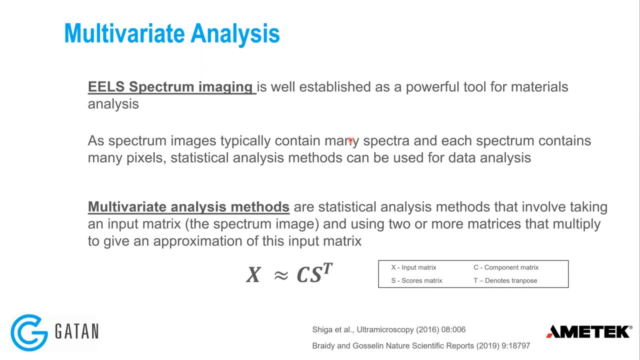 contains many pixels, We can treat these statistically. So we can do statistical analysis methods for data analysis. So multivariate analysis methods are typically statistical analysis methods that involve taking an input matrix, which is the spectrum image, and then using two or more matrices that multiply to give an approximation of the input matrix. 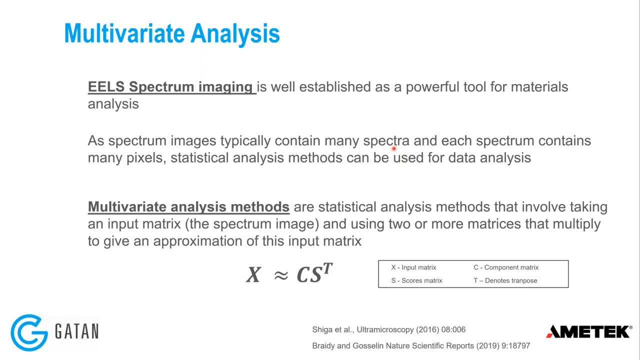 So this formula: here we have X, which is the input, matrix C is the component, matrix S is the scores matrix, And T denotes the transpose. So what does that mean for our actual data? It seems quite an abstract concept at the moment, So I'm going to limit this to kind of a more hands-on description. 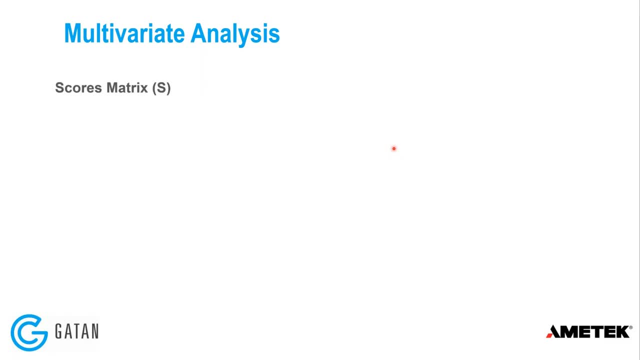 So I'm not going to go deep into the maths for the PCA. So in the scores matrix each row vector is a basis spectrum. Each vector is a basis spectrum. So in the scores matrix each row vector is a basis spectrum, Or what we call a loading. So that means the chemical phases represented in the data. 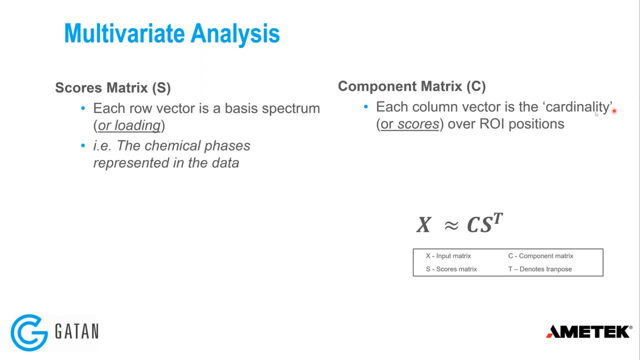 The component matrix, so the C matrix. each column vector is the cardinality, or what we call the scores over ROI positions. So that's really telling us the spatial distribution of the identified chemical phases. So we have one matrix, S, which tells us what we have like the different components and the other 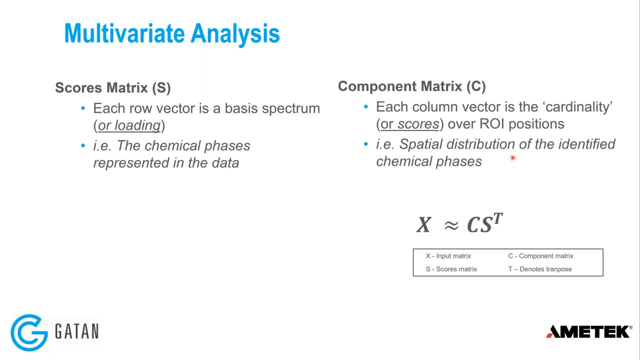 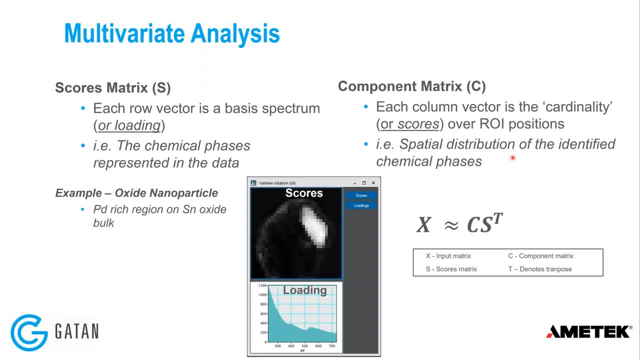 matrix C tells us kind of how those components are distributed around our sample. So let's look at a real sample and kind of see what that actually really means. So I've got this example here, which is a tin oxide nanoparticle. 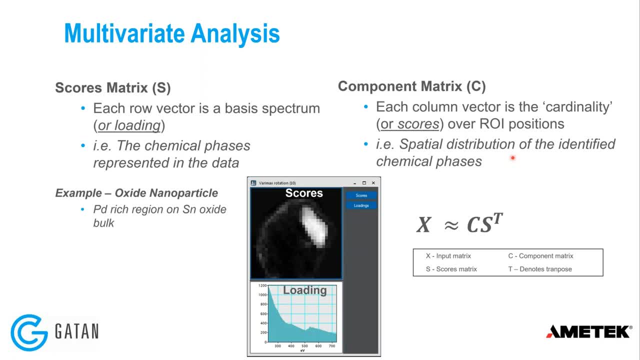 So this is an output from a Varimax plot. We're going to cover that later, but you can see that the top image here in this data set is the scores and the lower one is the loading. So the loading is the scores. 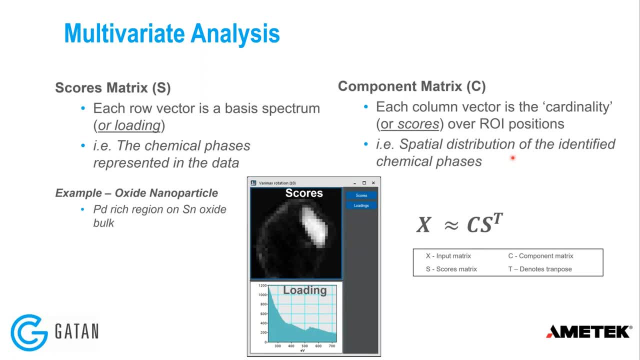 So this is the scores And the lower one is the loading. So the loading is the scores over ROI positions And the lower one is the scores over ROI positions, just kind of a spectrum, and the top is just the spatial distribution of that spectral component. 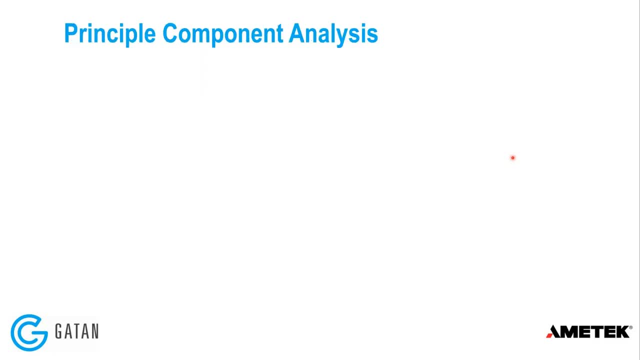 so that's, that's really it. so what? what about principal component analysis in particular? so principal component analysis is a particular flavor of multivariate analysis. so principal component analysis computes a projection that maximizes the total variance in the projected data. it casts basis vectors and score images in order in order of significance, so the more significant. 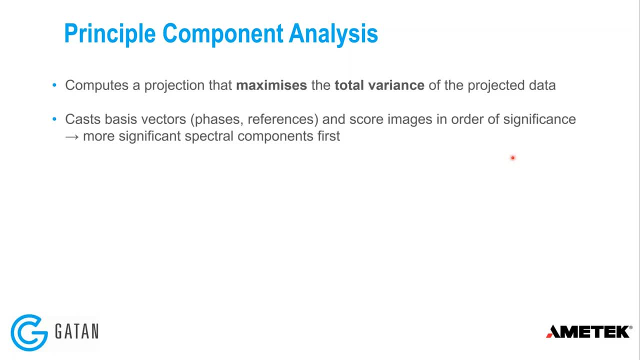 spectral components come first, which is actually quite useful in interpreting the data. the basis vectors are orthogonal, so this means that the spectral components are taken to be linearly independent, which is an important assumption. so typical applications: data mining, phase identification, phase analysis, noise filtering and data compression. 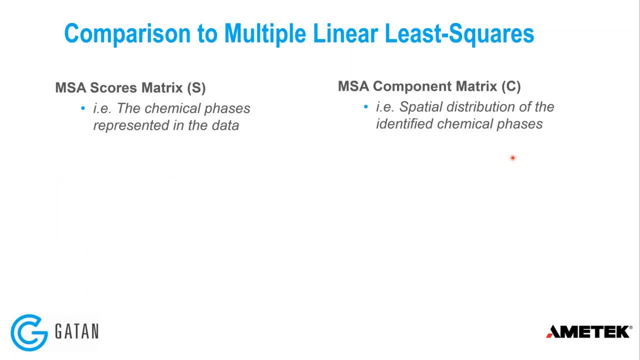 so we can make it, we can draw a comparison to multiple linear least squares, which is it's kind of nice. so if we have our two matrices, so we have our scores matrix and our component matrix, so the scores matrix in pca or msa is equivalent to the 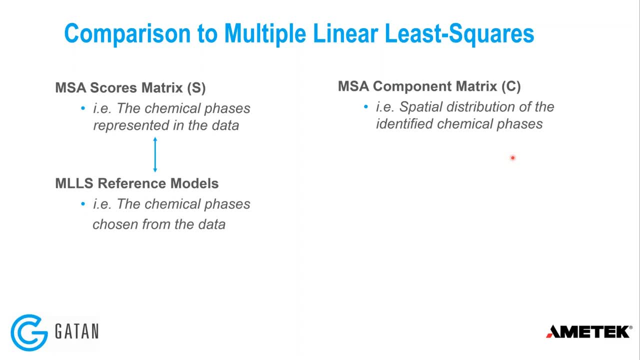 reference models that we're using in multiple linear least squares fitting. the component matrix is equivalent to the scaling coefficients that we have in multiple linearly squares fitting. so how much of the phases and where they are. so pca models the data as a linear combination of components, just like multiple linearly squares fitting. but there's a key difference, unlike in. mlls. we don't choose the components in advance, so the pca algorithm will just will choose the references that are statistically significant for us in advance. so there's a number of packages that exist that are out there. so axia from sandia, the msa plug-in for dm by watanabe from hrene research. 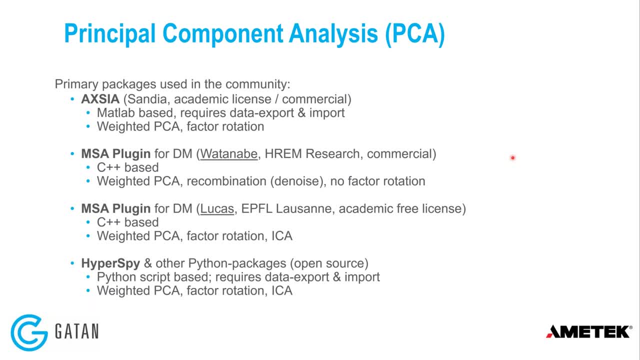 msa plug-in for digital micrograph that was written by the lukash group from epfl, hyperspy, other python packages. so some of these packages are free, some are not, and they have various different functionality like weighted PCA, factor rotation, denoising, etc. so I'm going to focus on this. this. 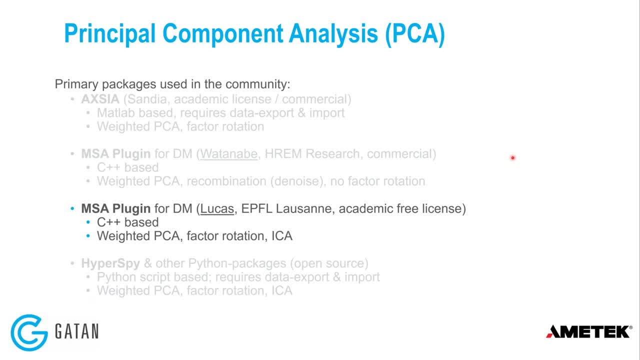 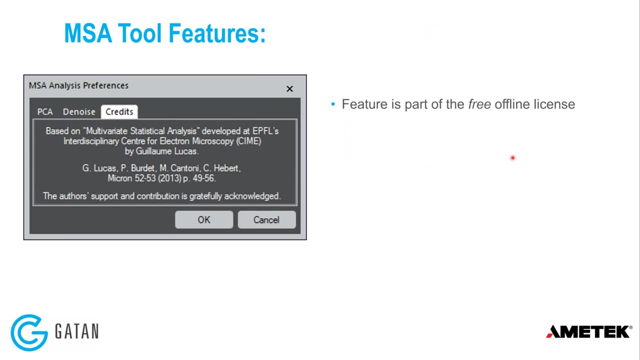 plug-in here, so MSA plug-in for DM by the EPFL group. so C++ based you can do weighted PCA factor rotation and independent component analysis. the reason I draw our attention to this is that this feature is part of the free offline license in GMS 3.4 and higher, so the the code that we have. 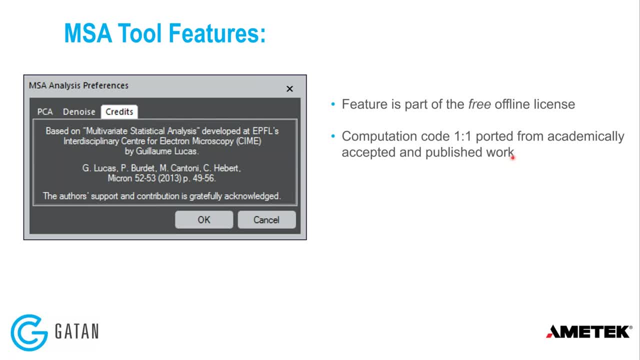 in our software is a one-to-one port from the academically accepted and published work by Lucas group, so we'd like to make a big thank you for those guys making the code available and allowing us to share it with everyone in the EM community. so what? the features of the tool. 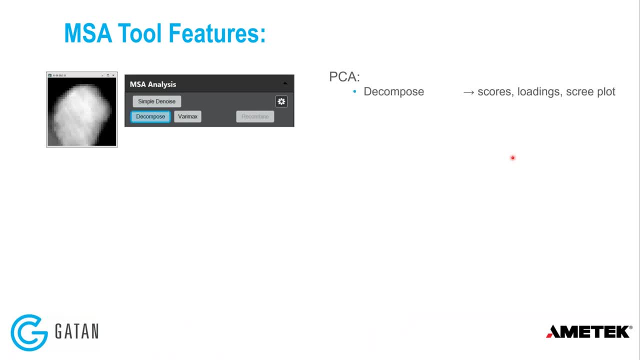 so we can do PCA. so we'll start off looking at the decomposition. so we have these three simple buttons, or four simple buttons. we're going to start on decompose. so if we run a PCA decomposition, we end up with a data set that has a score, the scores and the loadings which we just covered. 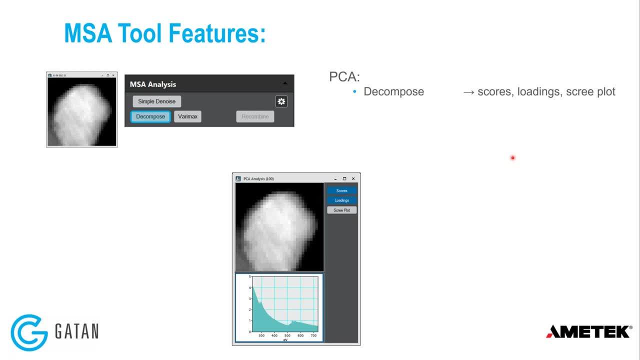 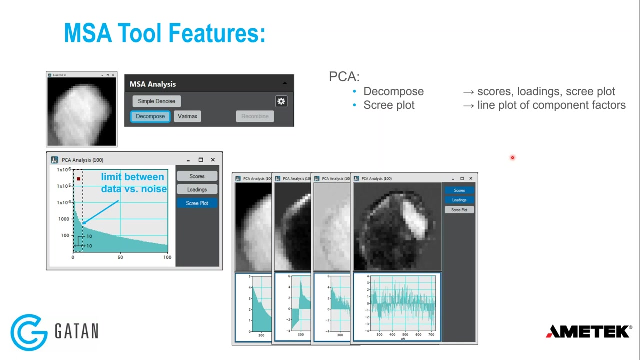 earlier and a scree plot, so I'll just cycle through some examples here. so here we're looking at the PCA components of this data set, so one, two in order of significance so you can see as we get to higher and higher components then kind of the variance is decreasing and that's really helping. 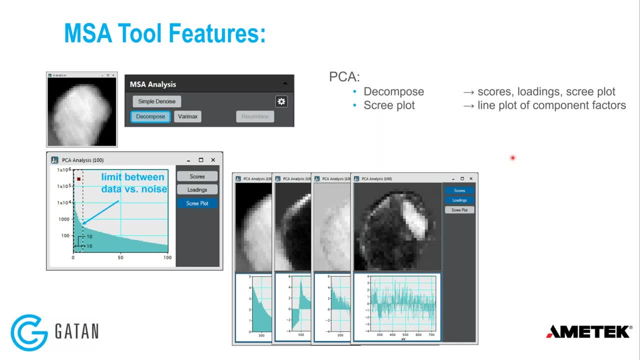 us interpret the data. so if we look at this scree plot, the scree plot is actually a line plot of the component factors and because they're in order of significance, it's super helpful for us to kind of make a decision between what's a real component and what's just noise. so if you look at the scree component, we typically the scree 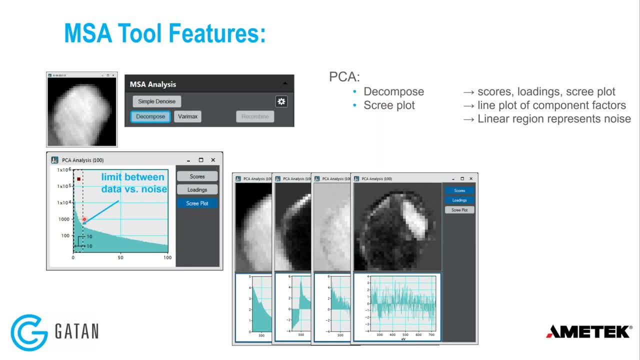 plot, sorry. we typically look for this knee or inflection point which is kind of telling us where our real data ends and the noise begins. so everything that's higher, basically in this linear region, we take as noise, so that's really useful. you can see in this, this plot, here we have 100. 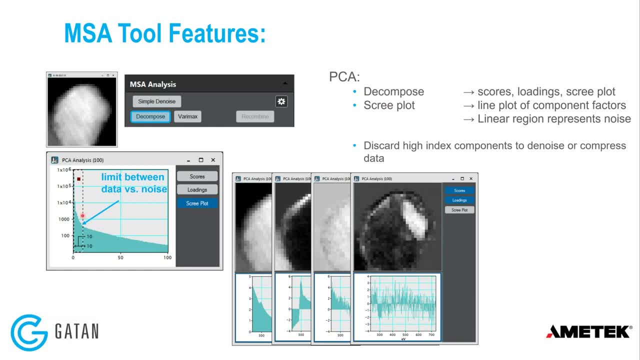 components, but it looks like only 10 are actual, real components, so we can get rid of the kind of excess components. so the 90 components that we think are noise, so that helps us because we're denoising. so that's the noise filtering aspect. we can also use it to compress the data, so we're reducing the size of the data set by a factor of. 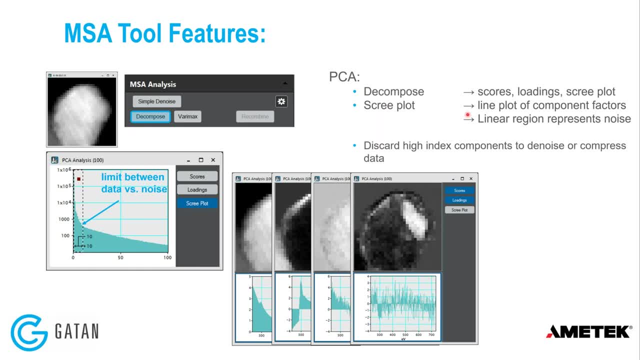 10, which is useful for processing, storage, etc. so one thing that is fairly clear when you look at these PCA plots here. but the variance was higher than the real data set. so we're really looking at, but there are regions that are negative, regions that are positive. so we have 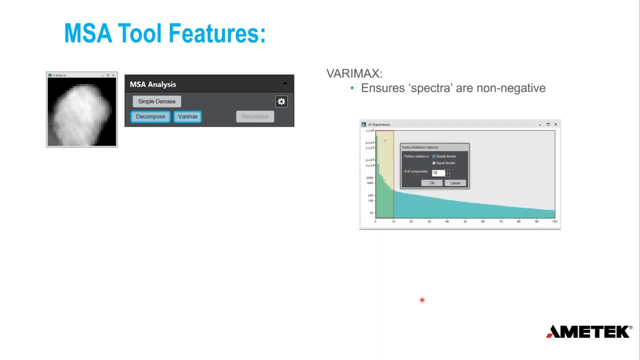 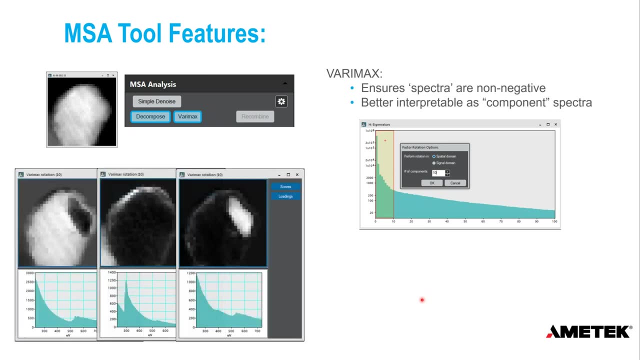 this other feature which is called very max. so very max basically performs some factor rotation to ensure spectra and non-negative, which means that the the results, the output are more interpretable as component spectra. so one thing to always remember is just, these are kind of, they're not net, not 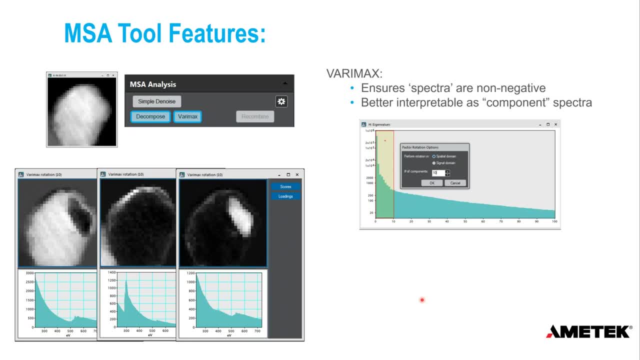 really real spectra. these are just, these are statistically kind of strong components in the data. so it's always worth kind of looking at the actual, real, the spectrum image data just to verify that we have components that make sense. it's kind of one final point: PCA, remember, is based on linear combinations. 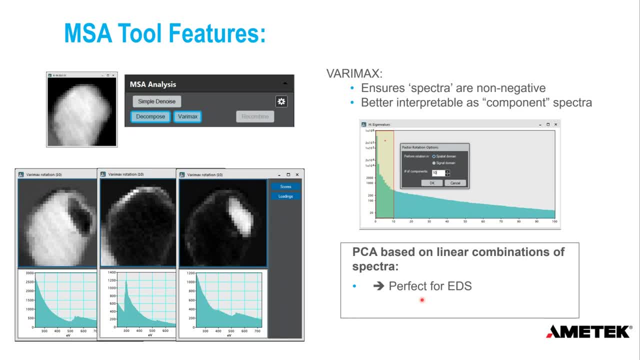 of spectra, and so that's really good for EDS. so in EDS we have linear independence of spectra, and so that's really good for EDS. so in EDS we have linear independence of spectra and so that's really good for EDS. so in EDS we 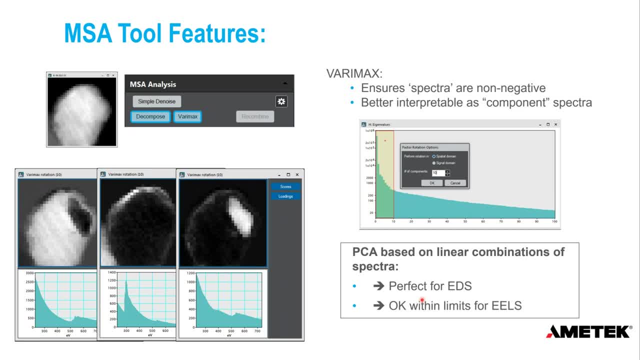 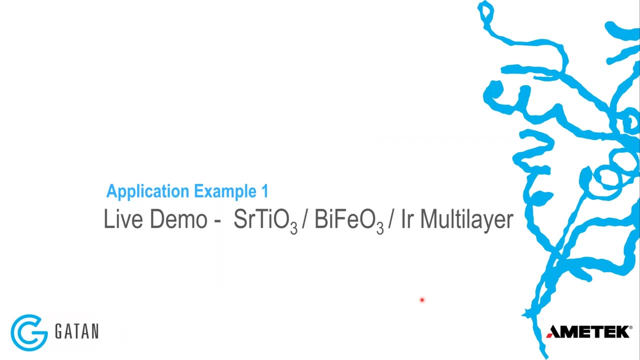 of our kind of peaks in EDS spectrum. that's not always true for EELS. so when we're doing PCA on EELS data, we need to kind of be a bit more careful about how we do the processing. okay, so that's a good point to jump to the software. so 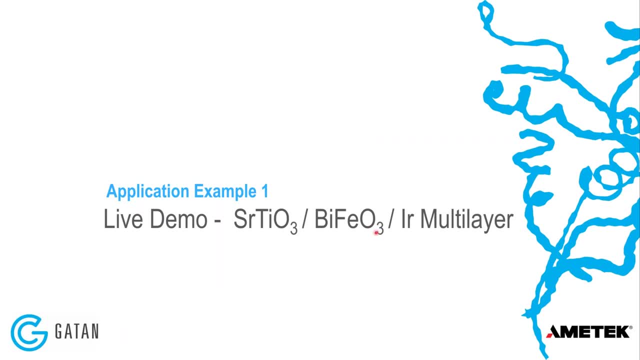 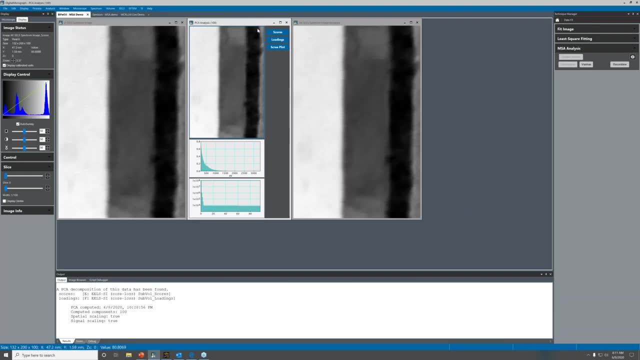 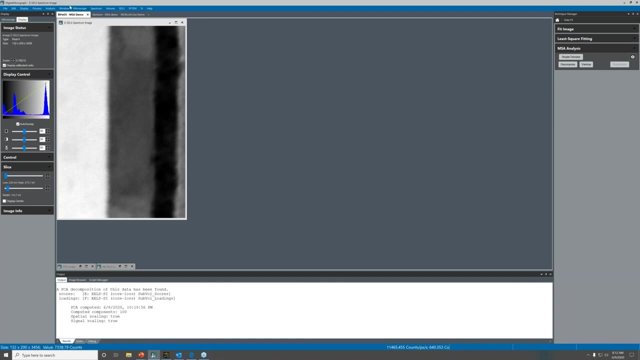 we're going to start off looking at this multi-layer sample. so I've actually already done that. so I've actually already done that. so I've actually done the decomposition on this guy. so this is spectrum image of multi-layer. so the the region on the left is strontium titanate, so that's a substrate. then we 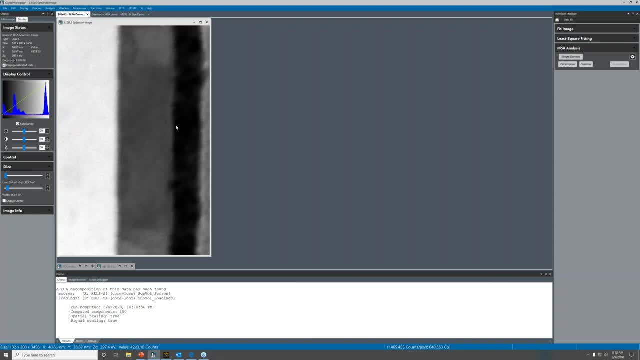 have a bismuth, ferrite layer, indium layer, and we have then platinum, so the platinum coating, so it's a fib lamella. So if we wanted to run a decomposition here, we would basically hit this week okay, so I'll exit. so if I exit, write out. 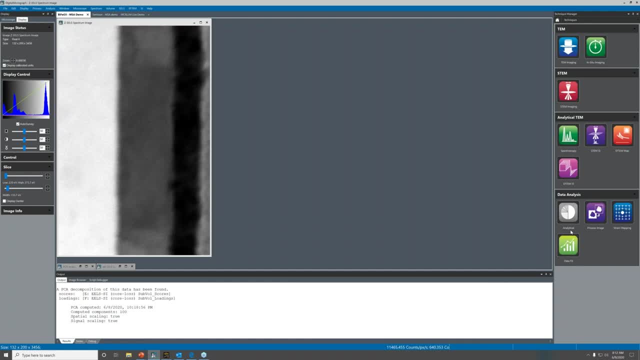 so the MSA tool is in the data fit data fit technique, which is in the data and analysis group of techniques. so I hit data fit and then you've got your MSA analysis tool here. so all the options are available here, because I already have run decomposition so we could do. 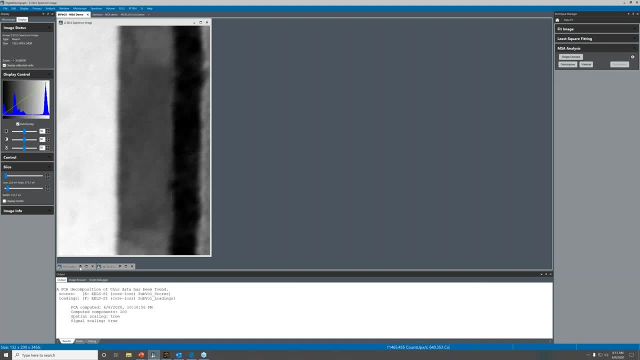 simple, denoise, we can do, decompose, we can do very max to save a little time. I'm going to look at the data set that has already been decomposed. so this is a PCA decomposition of the spectrum image so you can see straight away. I have three and three pieces of data in the PCA. 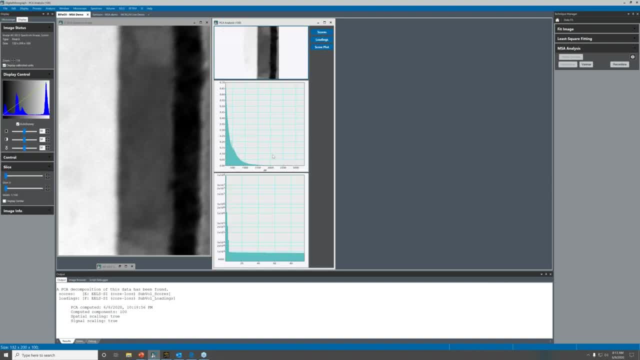 decomposition, so the scores, the loadings and the scree plot, so the way you navigate this data is used. select the data set and then we use the slice tool to kind of go through the components so you can see the first component, second, third, fourth, fifth, sixth and so on, and then basically 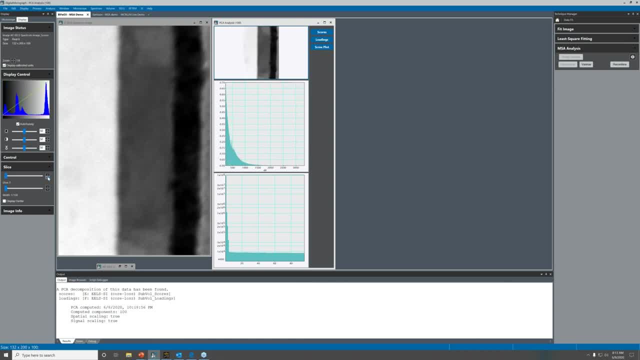 it's very clear with this data that the variance is high in these components. until about component component four seems to be the last real component and then after that we have this kind of pure noise component from component five. so if we keep going, yeah, you can see that it's pure Poisson noise. so this is a really well behaved data set. 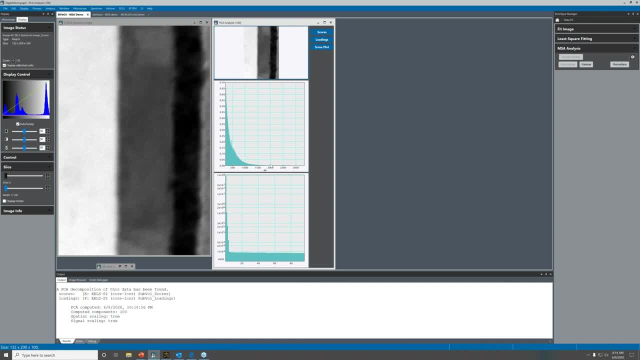 so we can kind of look at the scores, we can look at the loadings, we can also look at the scree plot. so so this is an example of a very easily interpreted scree plot. so this linear region is where we kind of we're expecting noise and we have a super sharp 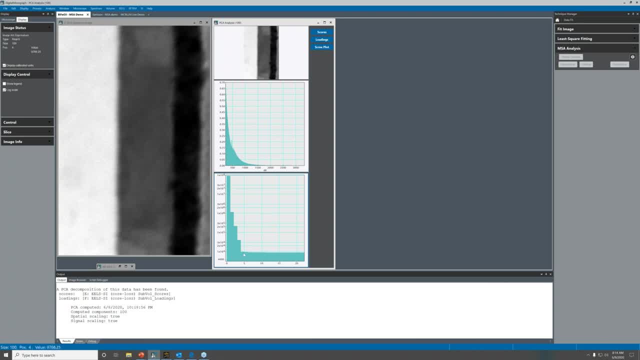 gradient and really strong inflection point. so it's like it's very clear that that is where we want to start throwing away our data. so so, yeah, so if you want to, we can do very Max, we can do denoise. so I actually already did a denoise. so this um is denoised. I kept. 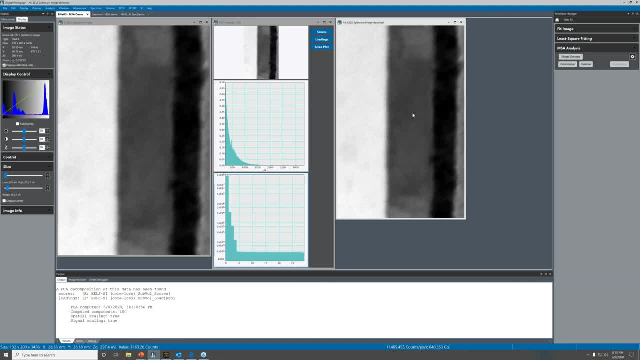 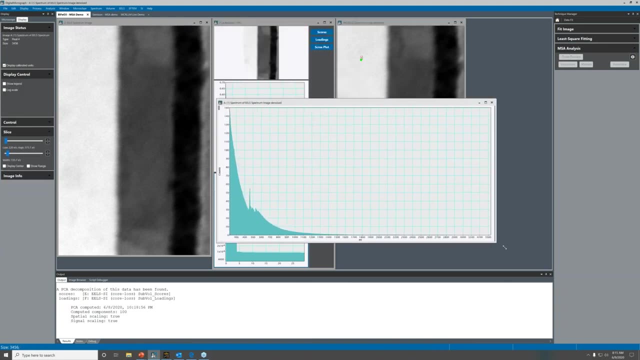 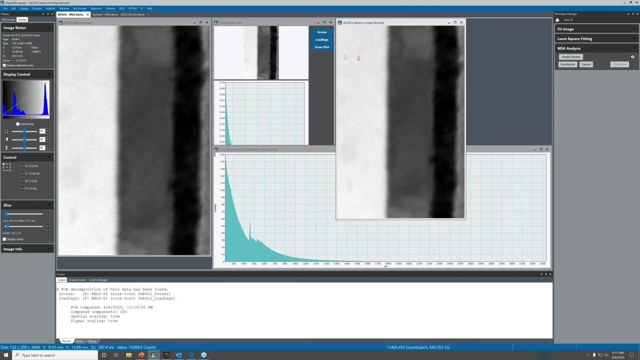 the four components. so there's. the four components are pretty much the sto, the uh- all right- the iridium and the platinum. so if I use a spectrum picker tool, pull out a spectrum so we have the denoid spectrum and I'm going to hold and drag that picker tool over to. 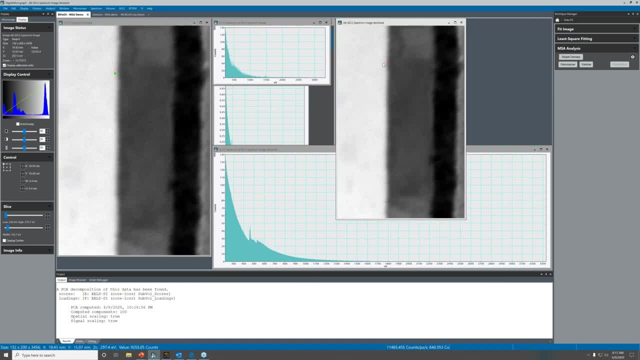 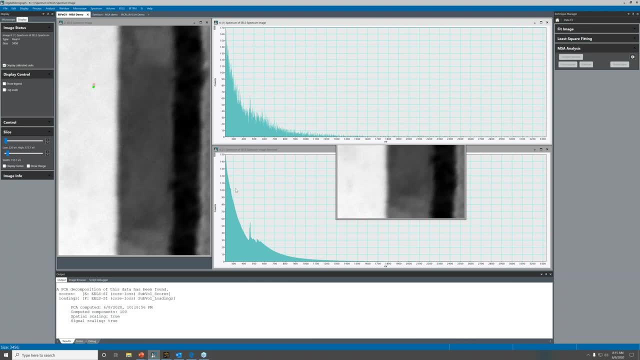 the original data. so the pixels are the same pixel. right, you can see the effect of the denoise. so it's very striking the effect of this denoise. we much, much clean, much, much cleaner data. so that's, uh, that's the first thing that we can do, simple denoise. 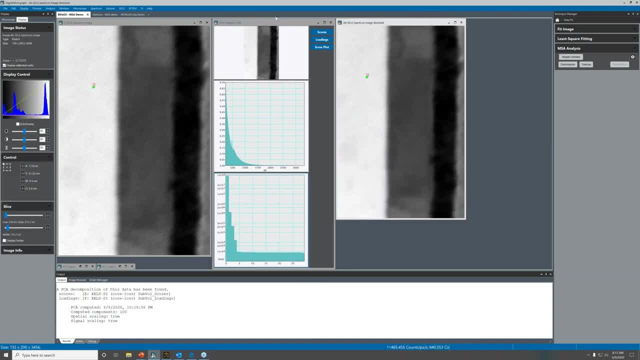 then let's go and do a very Max. so if you kind of again look at this guy, I'll sweep through the slices. why has it gone away? slice, okay. so remember we have strong variants in these components- well, the components that are real, but it's pretty hard to interpret what's going on. 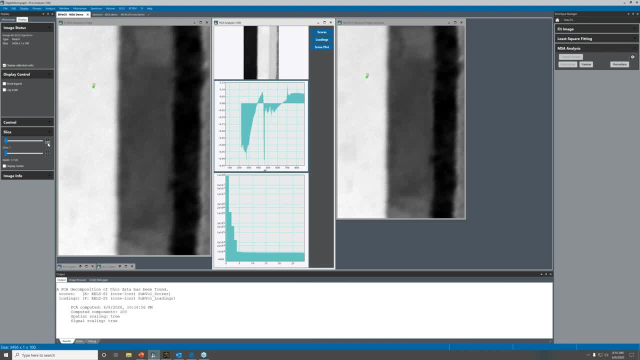 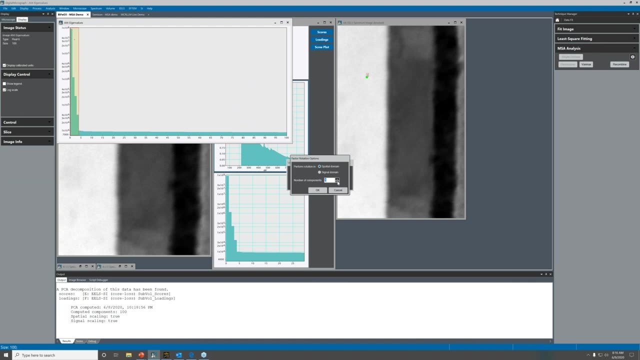 I mean it's like, yeah, that's a component, but what? what am I really looking at? loads of negative intensity. so we select the data set and then we go over back to the MSA analysis tool and we run very Max so choose the number of components to retain. we're going to perform the rotation in the spatial domain. 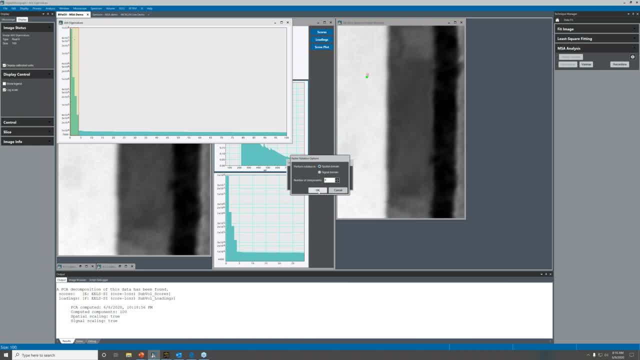 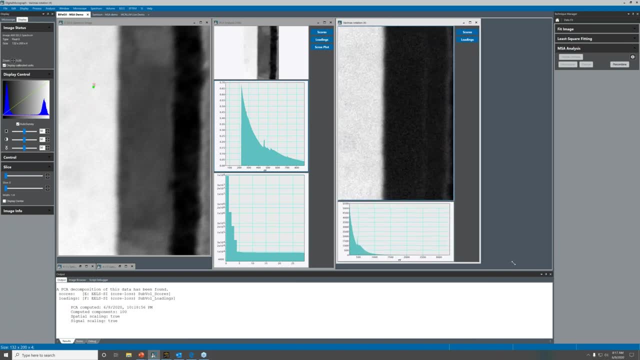 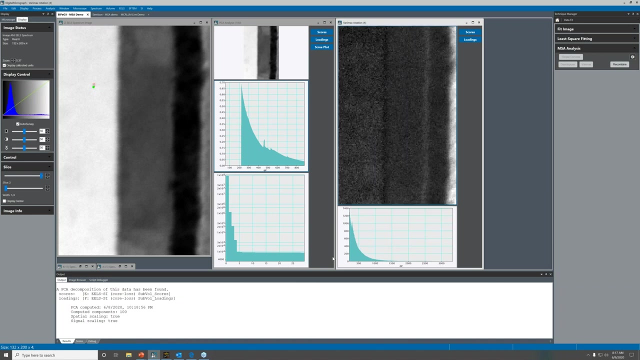 and then I hit, okay, okay, so let's put that data set there, okay. so now we have, um, everything's positive, right. so if we do the same thing, if we sweep through this and this components here, they're much, much easier to interpret what's going on. so 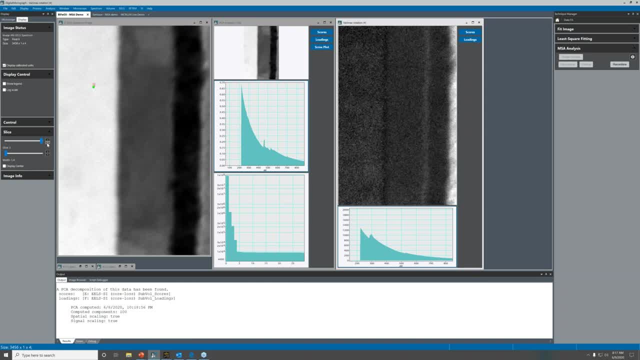 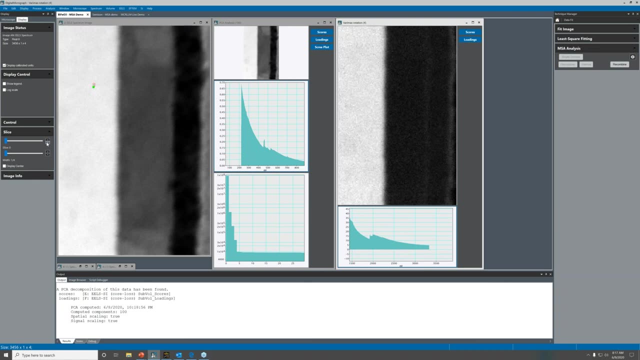 you can kind of see: oh, look there's, there's some carbon and there's some oxygen, um, iron, yeah, oxygen, and then there's some bismuth like way up high energy, yeah. so yeah, it's pretty nice way of kind of data mining, your data set and doing the denoise. 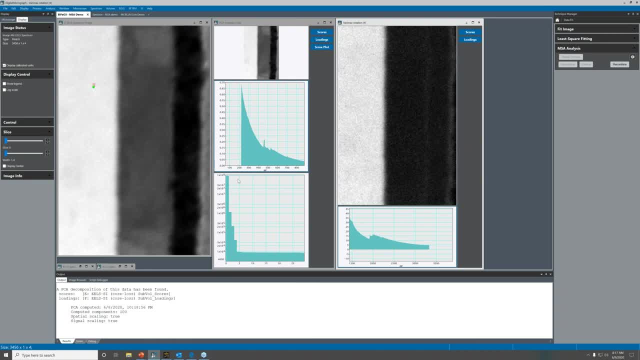 okay, so that's. that's an example of a sample that's pretty easy to work with. so this is counted data. this was from a k3 eel system, so we have very good, um kind of a very well-behaved detector. we have kind of ideal noise in the data and we also have a well-behaved sample. so this is a fairly thin. 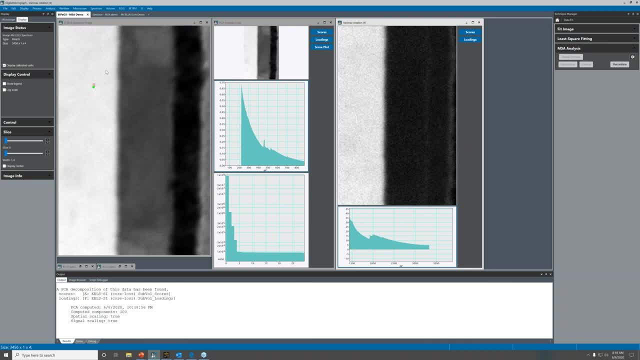 bib section, so it doesn't have any big changes in thickness. the plural scattering contributions are fairly uniform, so it's a combination of an. we have a good sample, but we also have a very good detector, so we're getting this benefit when we we're doing the analysis. so what about if we had? 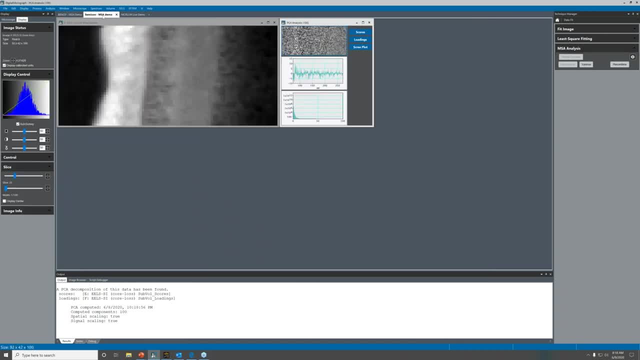 a data set that was a little bit more challenging. so I'm going to jump over to this semiconductor data set. so again, I've run the the decomposition already, but let's just run the decomposition again, because this is a smaller, smaller data set, so you can just see how how it runs. so we just basically hit, hit, decompose. I have the spectrum image selected. 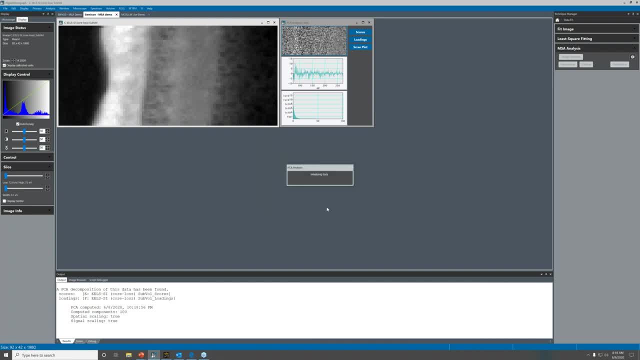 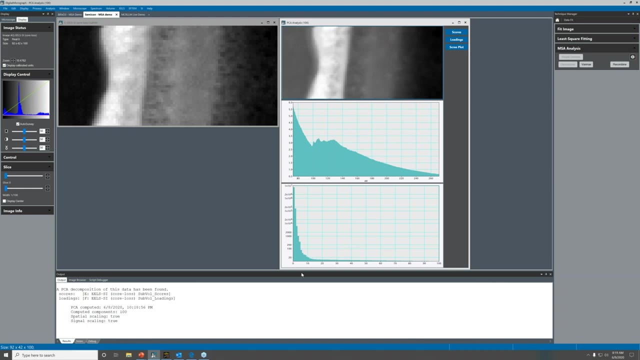 and I'm going to press decompose again. yes, runs the decomposition, so that's that, okay. so we end up with the same data. so we have score loadings in the plot so you can see straight away: um, with this data we have a much, much less obvious point. 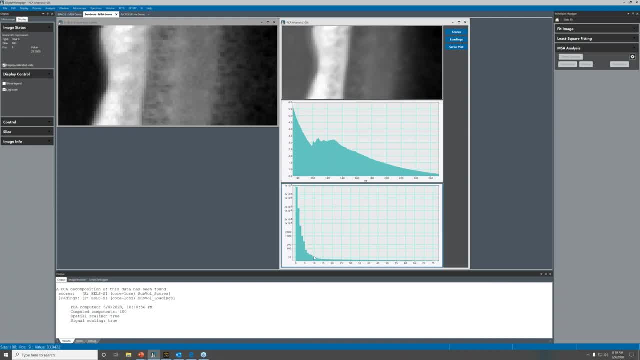 where we can say, okay, it's noise or it's real data, because the gradient here is: it's kind of a shallow change rather than a very abrupt, uh, change in the gradient in the screen plot. okay, so you might want to be a bit more conservative with this one. we could say, okay, let's. 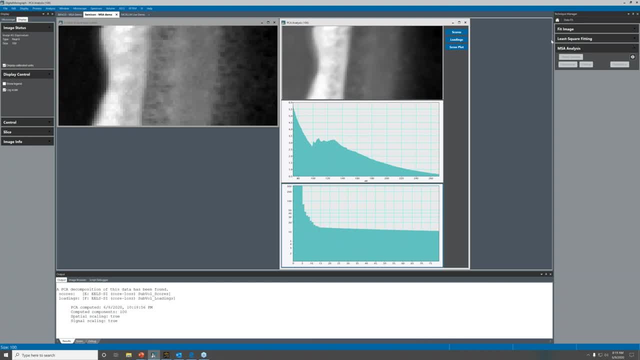 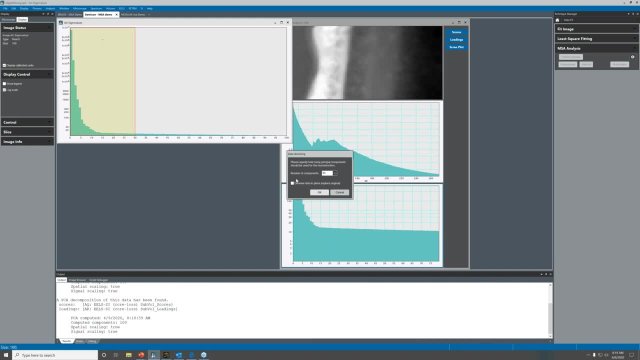 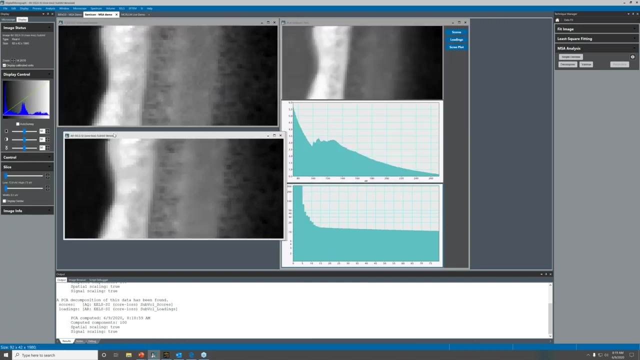 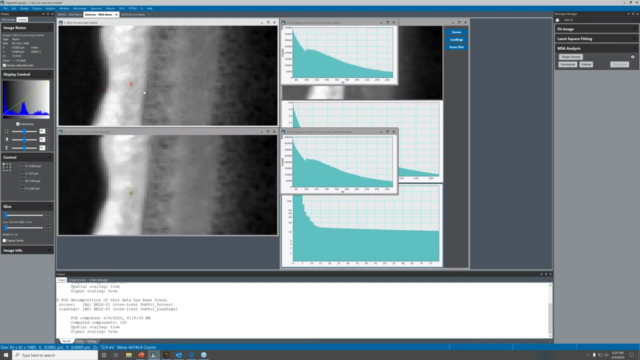 uh, maybe denoise to 15 components. so if we were to select this data, simple denoise, and then let's denoise to 15.. yep, 15, okay, that's the same thing. so we can do the same thing as we did before. so you can still see that. 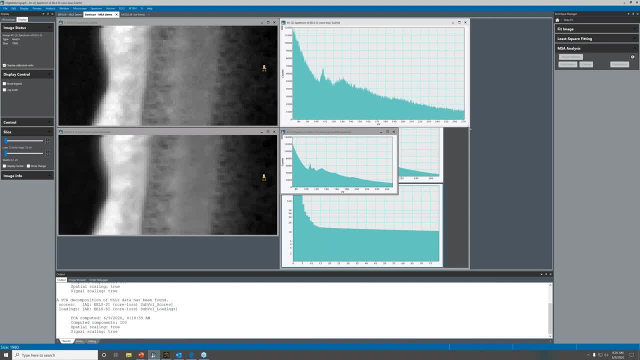 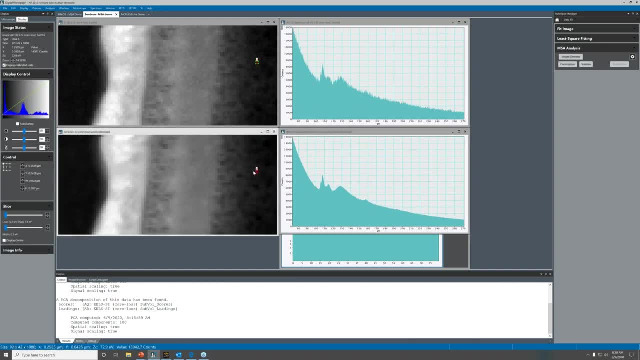 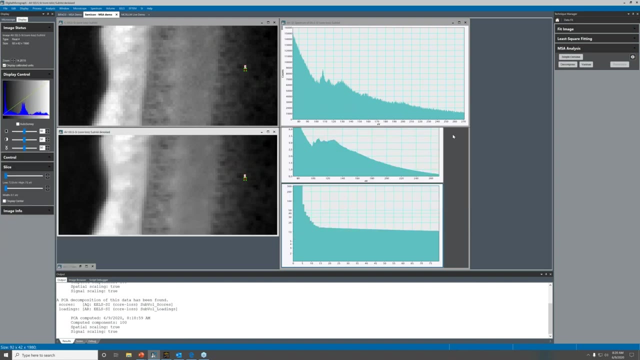 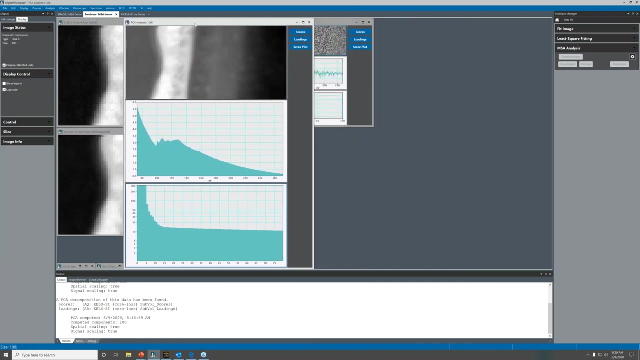 know, the top one here is the noise, the normal data set. bottom one is the denoise data set. so even with the fairly conservative denoise kind of still winning, which is which is nice. so yeah, okay. so with this data it's kind of more useful to kind of actually look a bit closer at what's. 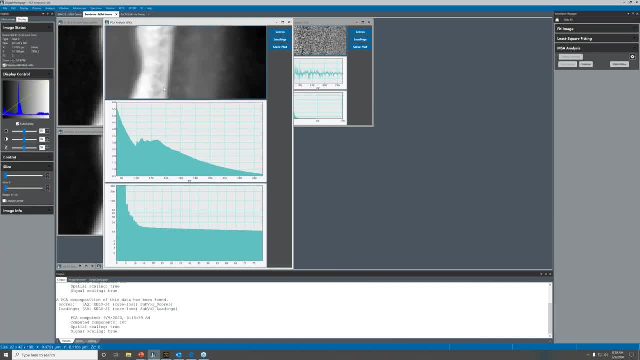 going on in the data. so we use the slice tool. again you could say, oh, I just denoise to 15 components, then maybe there's 15 components, but if you actually look at the day, so we again we start from zero. look at the variance in this. basically, we want to look at the structure in 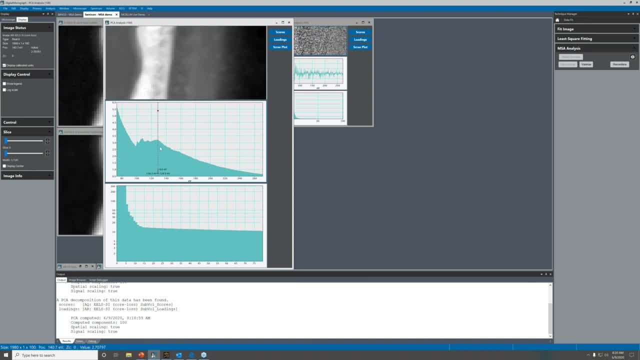 the scores images and you want to look at kind of the shapes of the of the loadings, so okay, so strong variance, strong kind of structure in this guy. little scores okay, so five maybe, but then as we kind of go a little bit higher, we do have kind of strong. 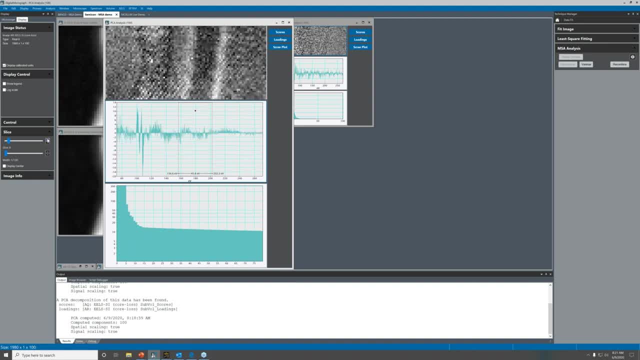 variance, but it starts to. it doesn't look like actual, real spectral components, so it could be non linearity in the deck in the data. maybe the thickness is changing. we've got some energy drift. it's just to do with the detector, the behavior. so you can see it looks quite different from the k3 data. okay, so let's. 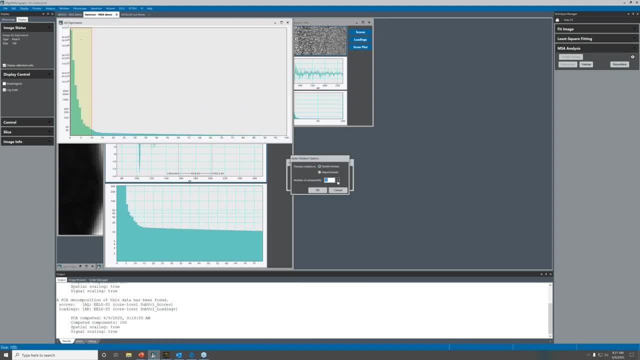 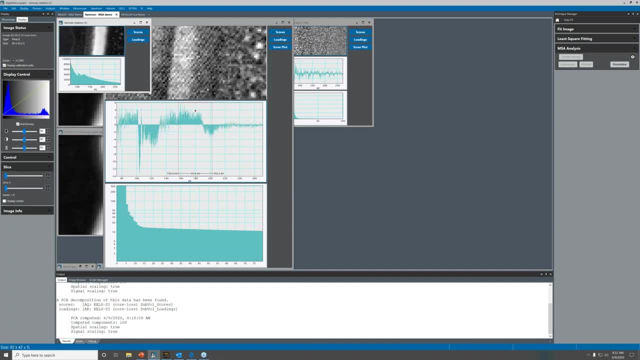 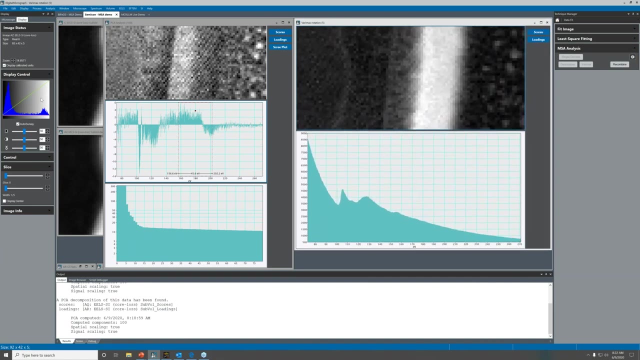 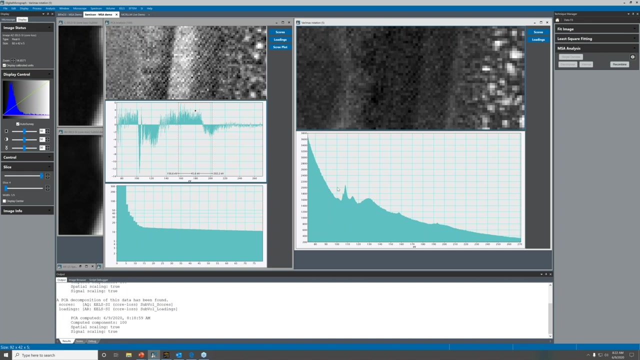 do a very max with this one with five components, okay, and then we end up with something another very max, another factor rotation, yeah. and then we end up with some nice, some nice maps and some. we've basically got, yeah, five different kind of spectral signatures for the silicon l23 edge in this sample. so we've got. 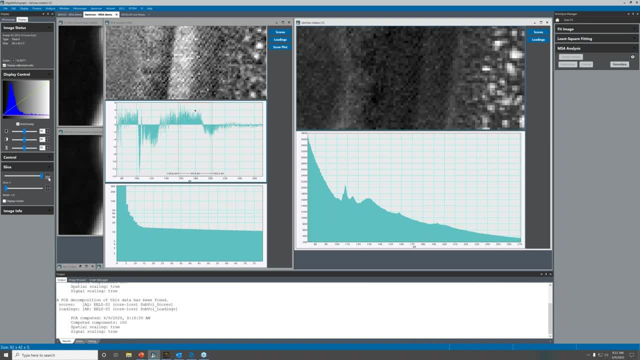 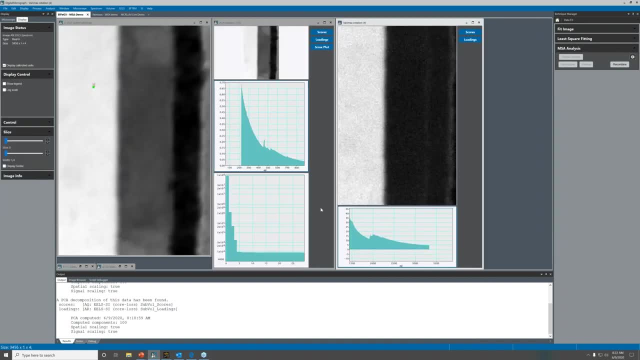 different layers, kind of these little precipitates and that's what we end up mapping. so you can kind of see from this, from from the other example you might think I could just I don't even need to look at the components, I can just from the screen plot, I can decide where to make my decision. but for 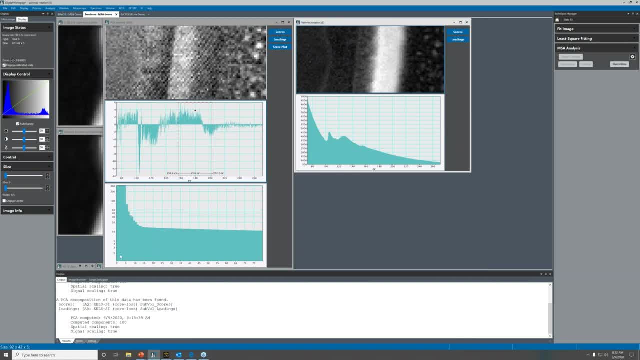 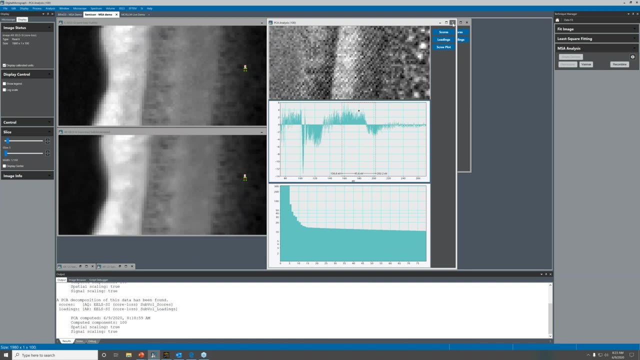 something like this that's a little bit more less sharp. it's kind it's important to do the decomposition, actually look at the scores and the loadings before deciding where to do your very max rotation or your d noise, for example. it's kind of one final thing that I want to show you with this. 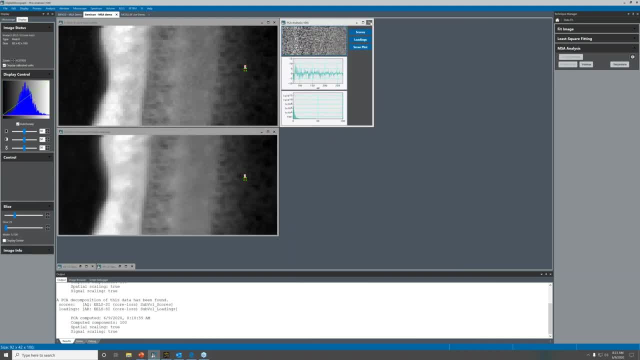 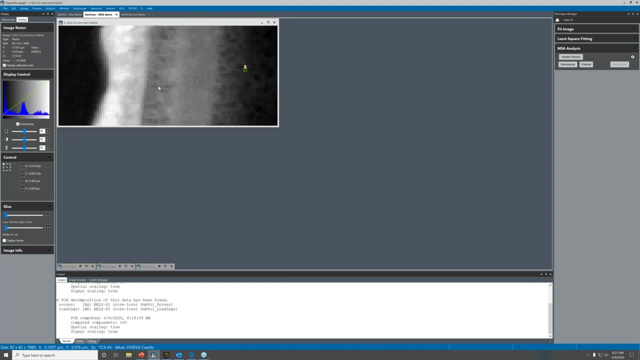 is that if I close everything, so if I select my original data, I've just thrown out the all the decomposition so that it's actually possible to run a simple d noise just as a one click option. so if we do a simple d noise, it will do the decomposition. 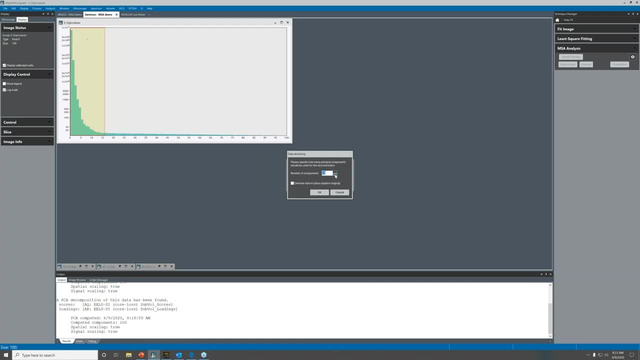 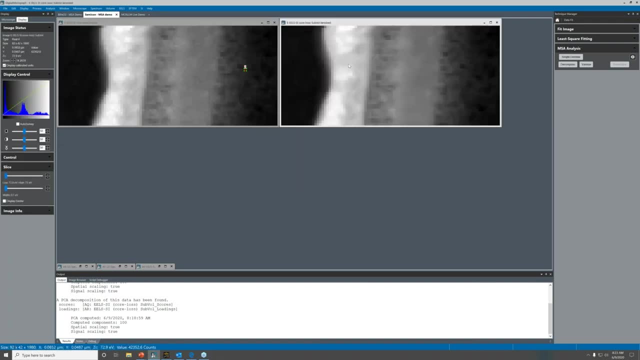 and then you can then say: okay, I want to d noise to 15 again, we'll do the same thing. so that's, that's really nice. that's a very quick and easy way to do the simple do do a d noise. but bear in mind, when you just do the simple d noise without the 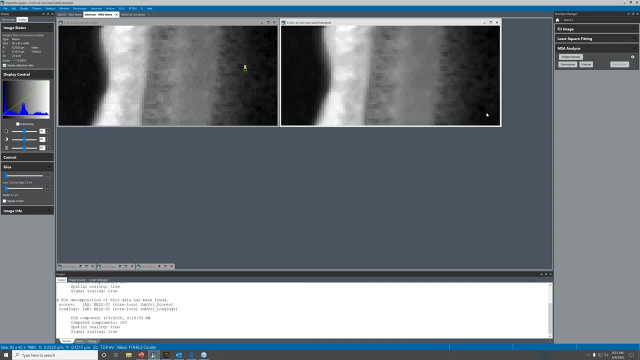 decomposition. it's not keeping the decomposition. so if you're confident in the in, in the point in the data, that you want to kind of throw away components, simple d noise is nice because it's faster, but if you kind of want to dig a little deeper into the data, it's worth doing the. 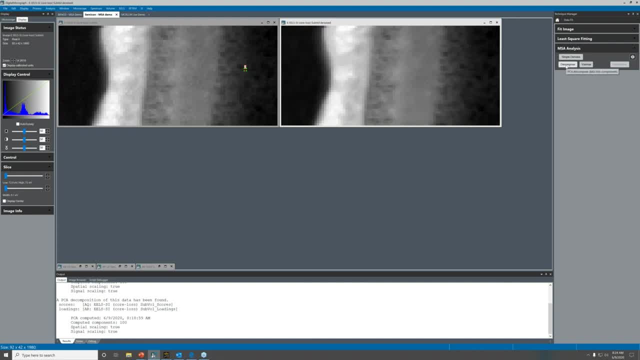 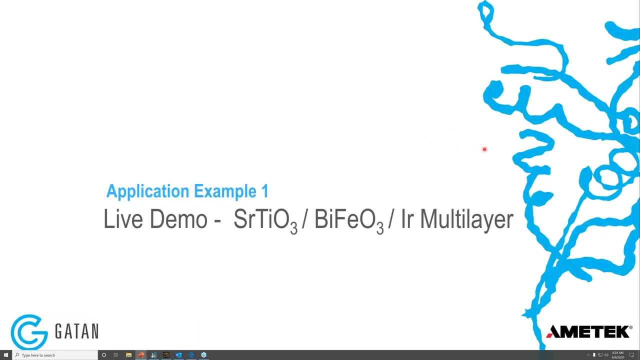 decomposition first, because then you can actually look at the scores, you can look at the loadings and then you can d noise after anyway, so you have the two options, two options there. okay, so pretty much covered that. so let's go back to the webinar. okay, so there were actually two, two examples there instead of one. okay, 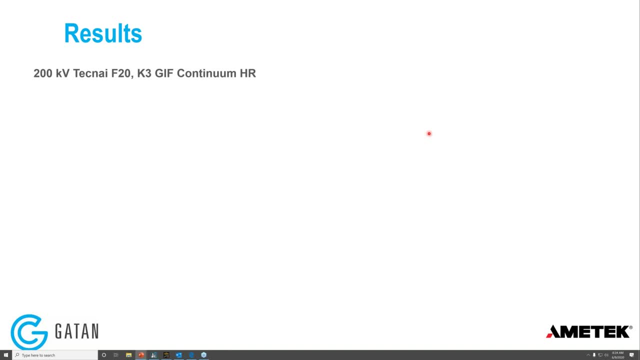 so I compiled the results from the k3 data onto the slide to make it a little nicer. so I got the data and then the��디 presented it so that data was actually taken on a techni f20 in Pleasanton. so it was done at 200kV, 0.9 Ev per channel dispersion and each pixel was 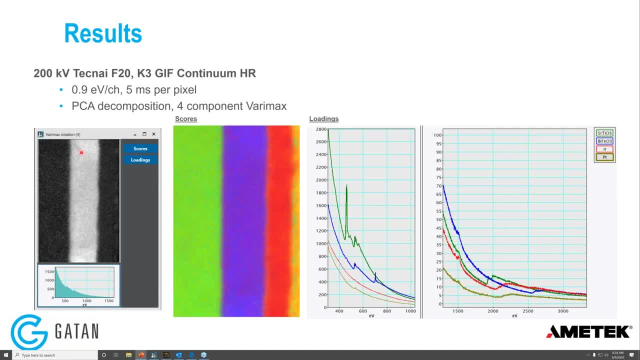 five milliseconds. so we did a pca decomposition and a four component, varimax. so this is a color mix of the four components. so green is the bismuth ferrite component. oops, no, it's not strontium titanate. green is strontium titanate. 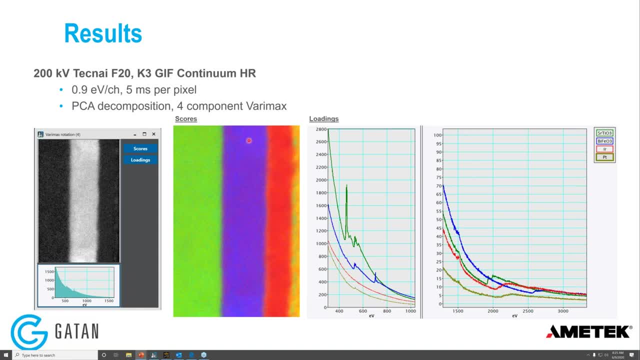 oops, no, it's not strontium titanate. green is strontium titanate, blue is bismuth ferrite and red is iridium and yellow is platinum. so you can have the scores overlaid and make a nice, nice color mix, and then you can also pull out the loadings and make like a waterfall plot or 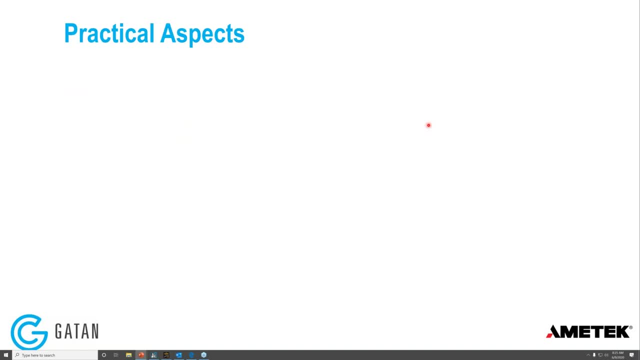 whatever. so it's a nice way of presenting the data. so now let's kind of go into some practical aspects. so it was kind of starting to become clear when we looked at the software live that you need to take care interpreting the scree plot. so this is the same scree plot that we just saw from the k3. 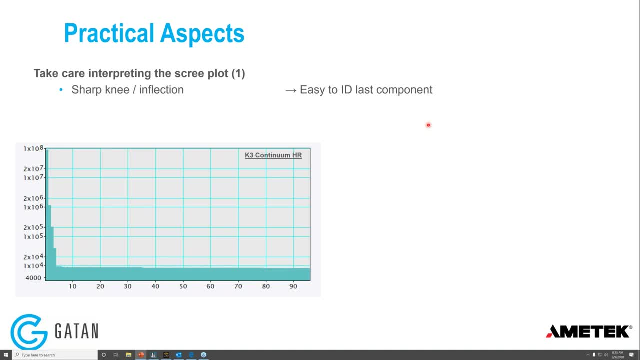 data. so when there's a sharp knee or inflection it's really easy to id the last kind of major real component. but if it's shallow change or there are multiple inflections it's a bit more difficult and therefore easier to miss real data. so let's take a look at the screen plot. 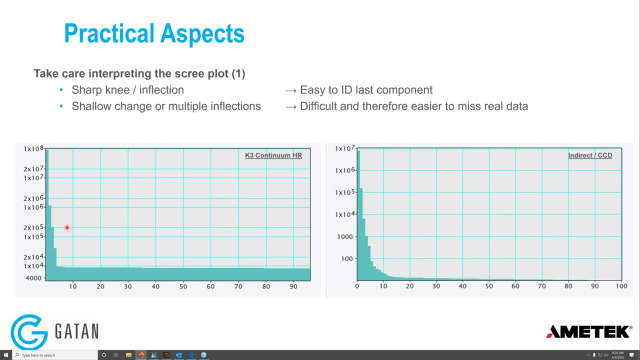 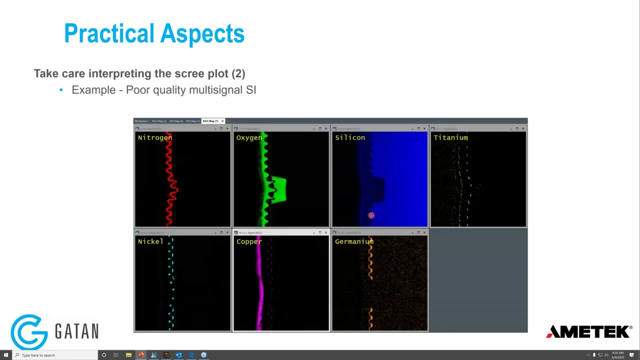 data. so this is kind of an easy case. on the left, the k3. this is kind of like as a medium case. so this is more challenging, but it's still not unreasonable. but then we're going to now look at something that is much more difficult. so we have an example of a quite poor quality. 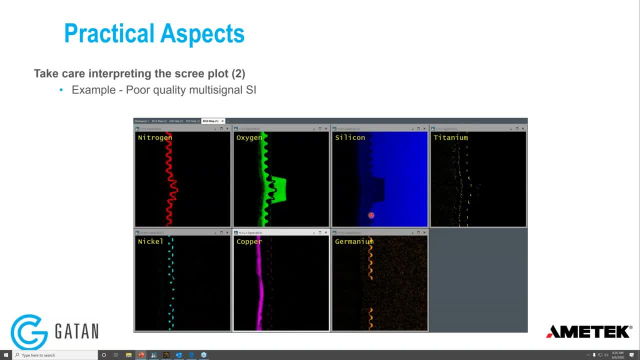 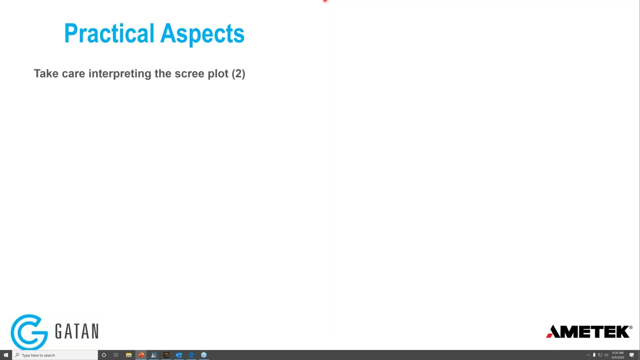 multi-signal spectrum image. so we were doing eds and eels here and we found that the video was actually quite good but it was not working. so we designed a much more complex model and we made a very small choice and we thought, oh well, i don't need a screen plot, so we're going to go ahead and 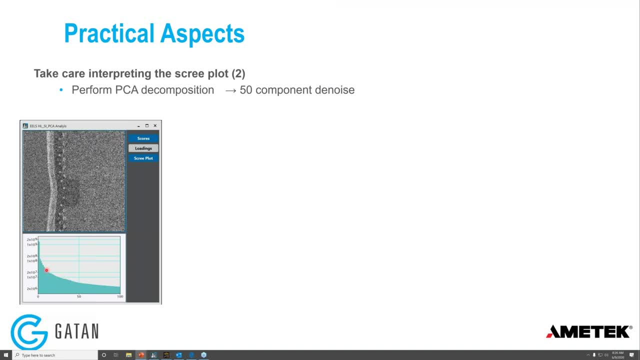 go ahead and make it into a believable model, which is actually a pretty nice kind of map. so we just moved it down to the left side of the screen and, as you can see, you can see that the screen plot is a bit more different. now. it's kind of that same screen model, but much more natural, and 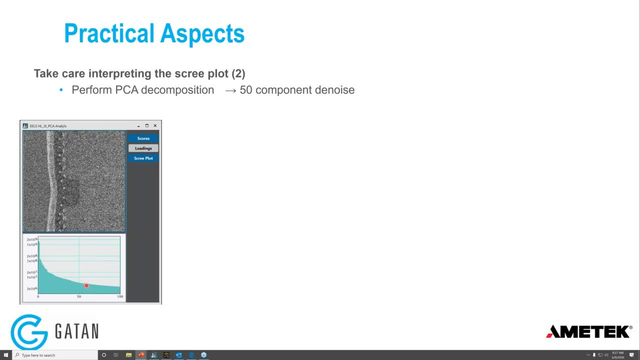 so and, as you can see, this is the screen plot right here and what this is about is. this is the screen plot right here. it's like the same value data. so now it's just a little bit different parts of the very much shallower kind of changing gradient. here it's saying kind of looks. 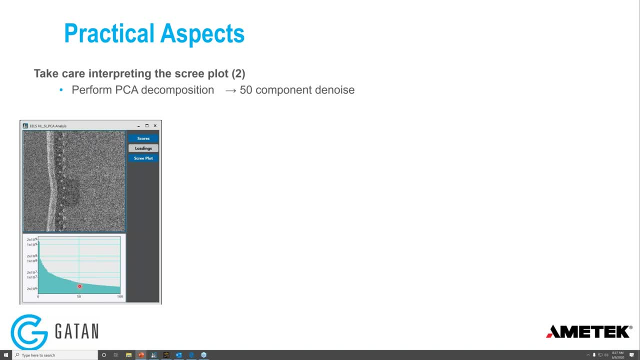 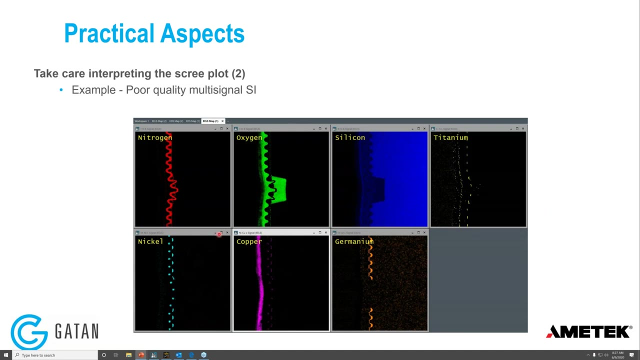 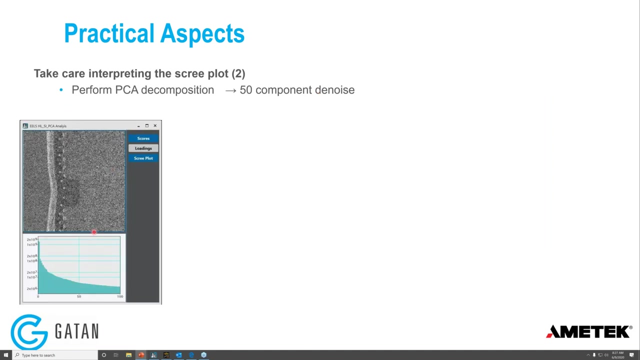 like it might be linear at 50 components and you could think, well, normally I throw out everything over four, five, ten components, and we can also look at these elemental maps and we think, well, I've got however many components, eight, no seven, so we got seven components. so we might think actually 50, 50 denoise with 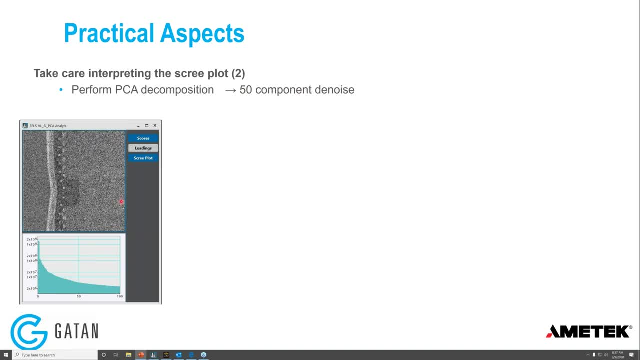 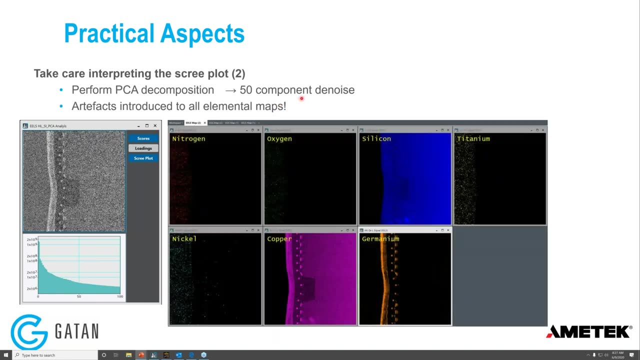 this data is very conservative because we've only got seven, seven actual spectral components, so it's fairly safe. but with this data it actually made the mapping worse. so if we look at the titanium, we don't have any titanium in real, real titanium information in our map anymore. oxygen nitrogen have changed. 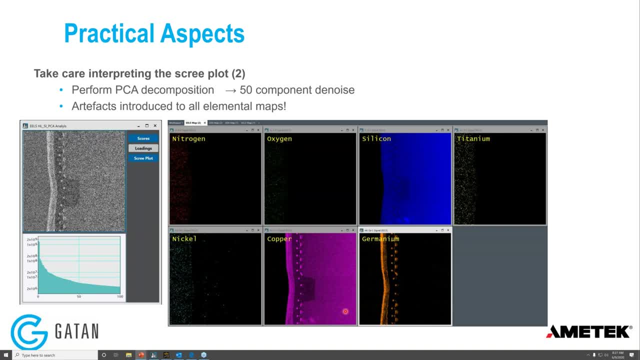 and nickels. basically every single map here has changed. so we've kind of naively thought that we would make the mapping, so we would do something about this. but the reality is, if we look at different systems we would have to make our maps better. but we've kind of we've 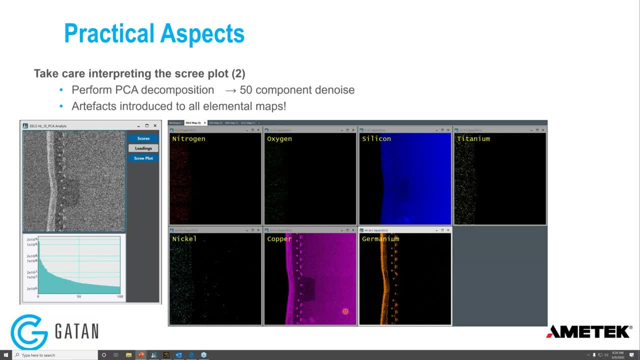 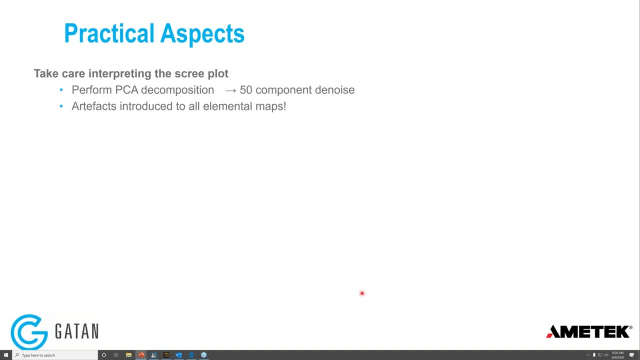 thrown out a load of information and then created artifacts in the other maps. so you have to treat the data with some sense and kind of you know, make sure that data is good enough to decompose in the first place. it's not a love easily on magic bullet that will make bad data into good data. so what else? and I guess 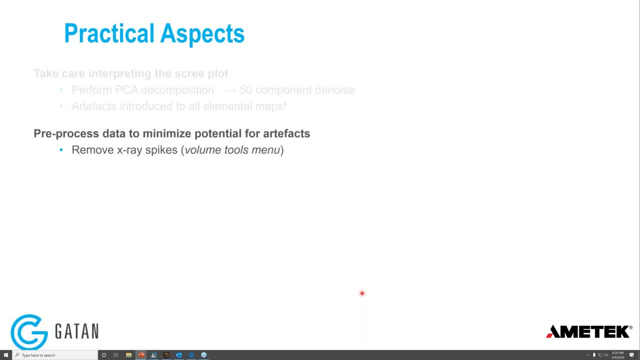 minimize the potential for artifacts. so it's always worth removing x-ray spikes. there's a simple one-click function in the volume tools menu, so always remove x-ray spikes before running MSA decomposition. consider deconvolution if the specimen has large change in relative thickness, and then you can also. 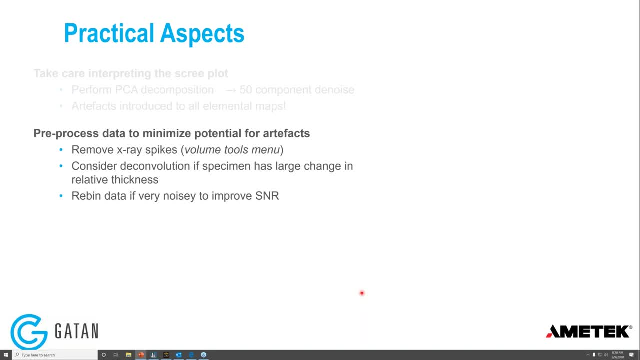 read bin the data if it's very noisy to improve the signal-to-noise ratio. so that's also possible through the volume tools menu. one other thing: the MSA tool is really good as a precursor for other automated analysis. so it's a compiled plug-in. it's written in C++ so it runs at relatively high speed on a fairly 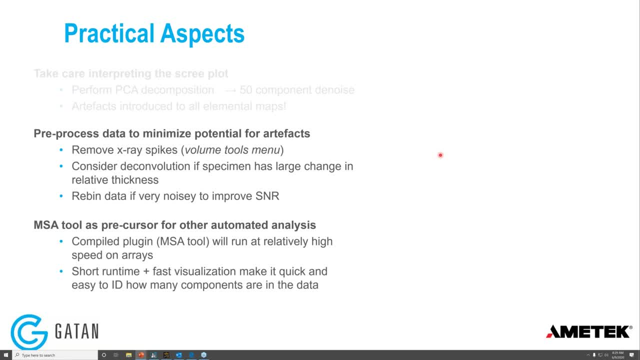 large arrays. it also has nice visualization tools, as you've just seen, so it can be a very fast way of kind of pre-screening your data, identifying how many components there are, and then you can- then you know- basically help yourself out. if you're running other automated analysis that's slower where you have to enter the 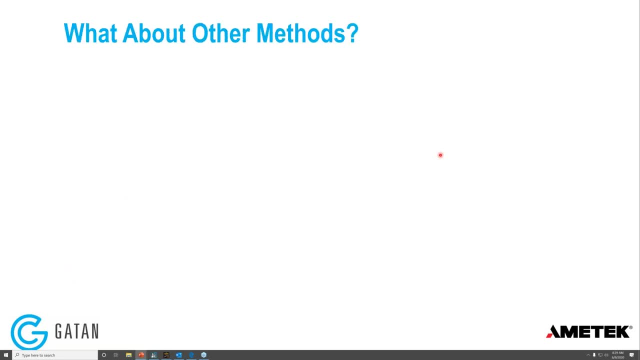 number of components you have. so what about other methods? so yeah, the big advantage of our tool is that it's an embedded tool in GMS so it'll run natively on any spectrum image data object you have in the software. you don't need to import, export or do anything funky with the data to be able. 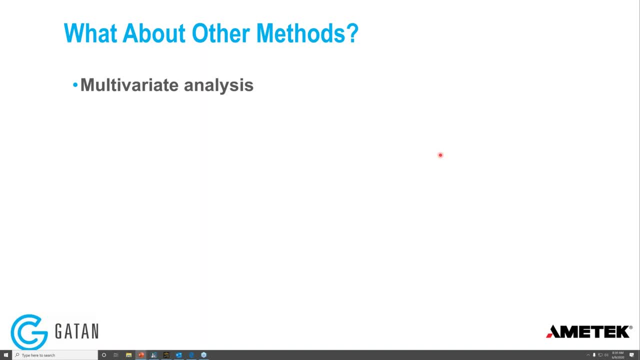 to do data. so it works very well with your and you know there's going to be new tools, new packages published, so if you want to use them, how would you do that? so that's kind of a nice segue into Python. so GMS has always had its own scripting language, which we call DM. 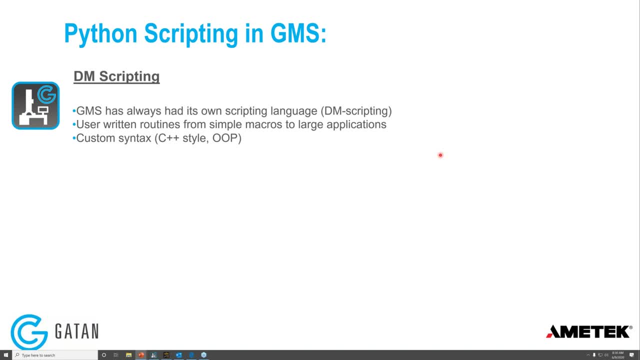 scripting so you can make user written routines from simple macros to large full-scale applications. has a custom syntax built on C++ and you can do object-oriented programming. Python is the fourth most popular programming language and it's being increasingly used, as probably many people know, for 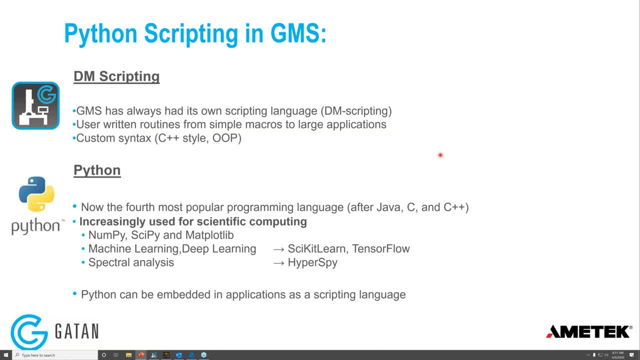 scientific computing. so there's loads of really great libraries like numpy, scipy and matplotlib. you can do machine learning, deep learning using scikit-learn, tensorflow, we can perform spectrum analysis, analysis and something like hyperspy. so Python can be embedded in applications as a scripting language and which we've gone ahead and done in GMS 3.4. so GMS 3.4 now includes Python as. 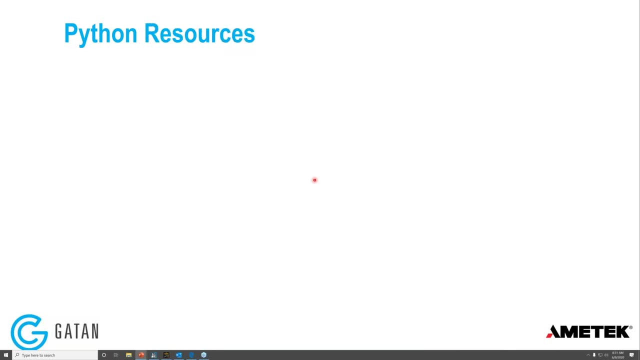 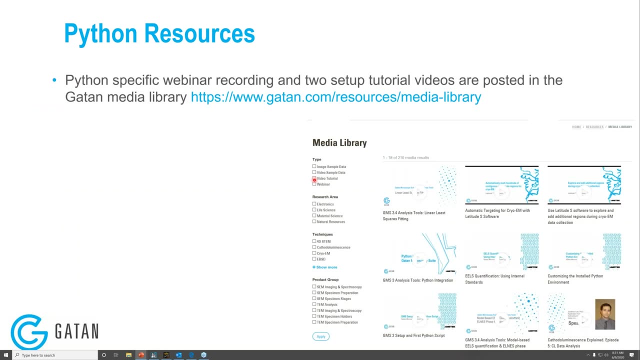 a scripting language, so we have some resources available on our website. so there's a Python specific webinar that Ben Miller gave a few weeks ago and there's a recording of that webinar on the media library, so the link to the media library is there. we also have two Python specific 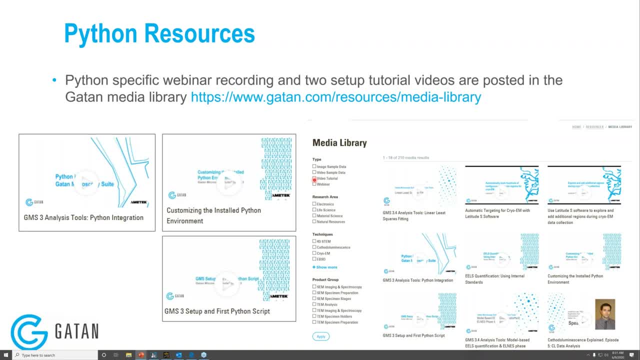 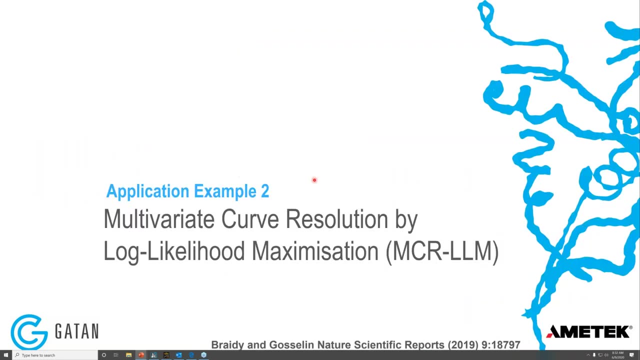 kind of short tutorial videos and kind of telling you how to get set up and how to install external packages. so if anyone's interested in getting up and running with Python scripting and hasn't seen that content, I'd recommend checking it out. so that's kind of a nice segue into 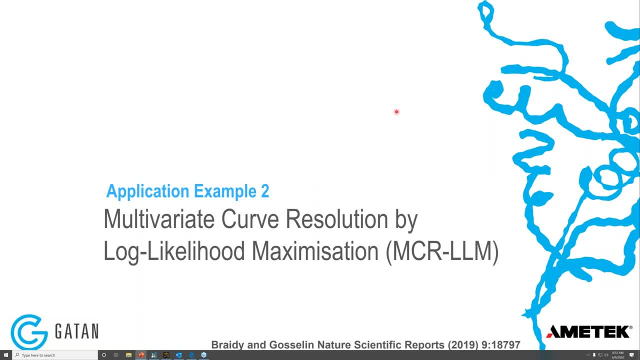 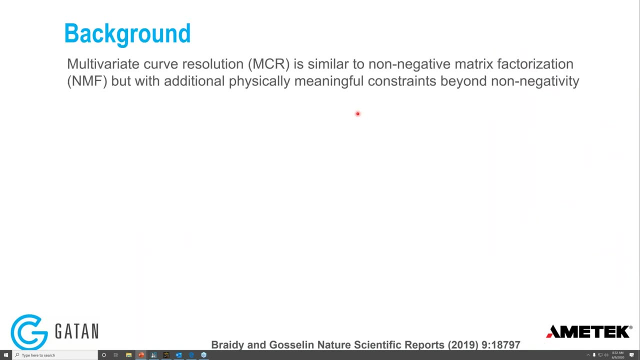 example two. so this is multivariate curve resolution by log likelihood maximization, or MCR, LLM, which is much easier to say. so some background. so multivariate curve resolution, or MCR, is similar to non-negative matrix factorization, but with some additional physical, physically meaningful constraints beyond just. 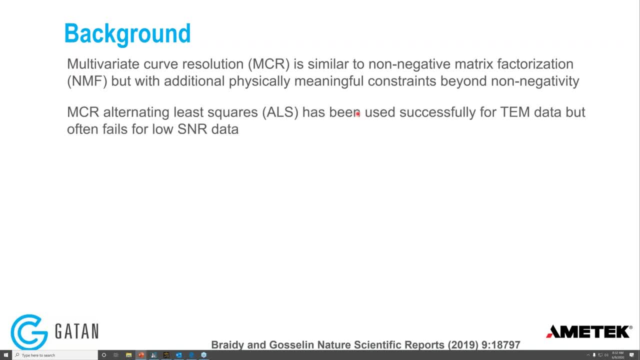 non-negativity. so MCR alternating least squares. so MCR ALS has been used successfully for TEM data and it's been used for a number of other applications. but it's often fails or gives funky results for low signal-to-noise ratio data. so professor Brady and Goslin and professor Goslin have used a Poisson. 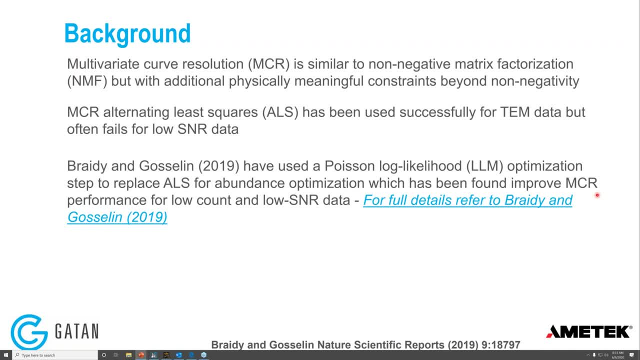 like Poisson log likelihood. so LLM optimization step to replace ALS for abundance optimization, which they found really improved MCR performance for low count and low signal-to-noise ratio data. so if anyone's particularly interested in that I'd be happy to help you out with that. 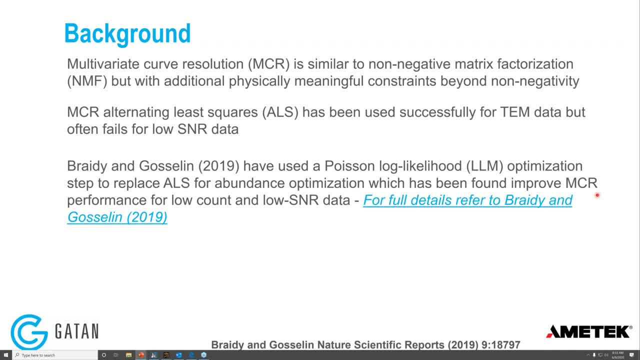 interested in the background and the theory in this method, I refer you to the paper, so the full details are in this 2019 reference and nature scientific reports, which is at the bottom of the slide. I'm really just using this as an example to show how you can do something kind of non-standard in digital. 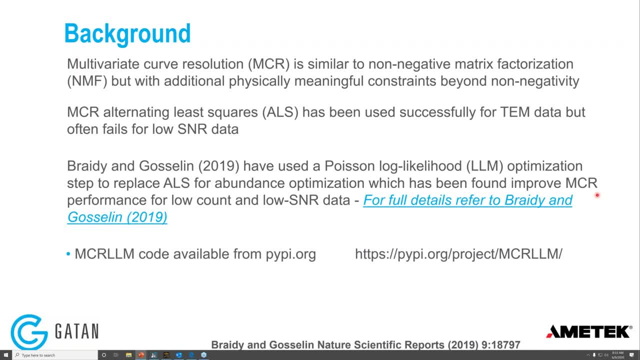 micrograph. so their code, their MCR LLM code, is available from pi pi org. so that's a link to code, and what's really great about this is that it's really great with this package and many Python packages is it's super easy to do the. 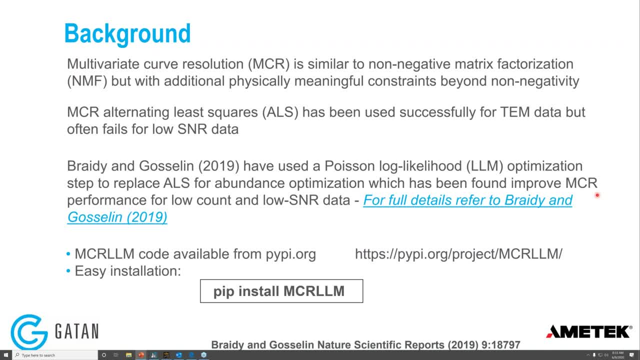 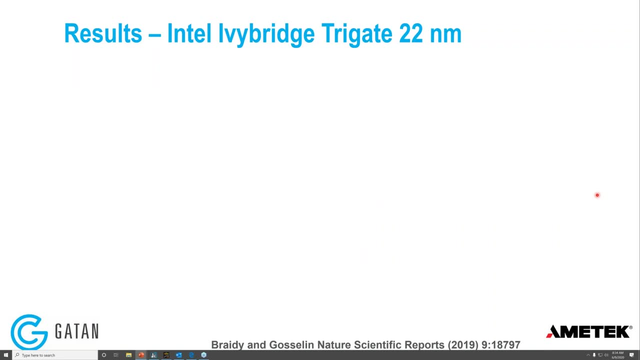 installation. so you just run your Python environment from a command line and you just have a one-line installation. so it's pip install package name, which is in this case MCR LLM. okay, so let's move on to some of the results. so they they have. 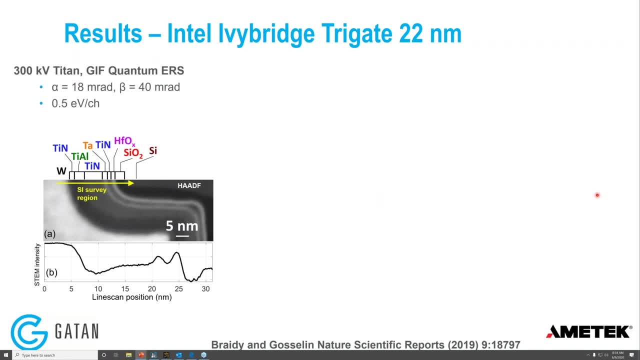 basically acquired a some spectrum image data from an Intel Ivy bridge sample, so it's a semiconductor, the gate. so they used Titan, so they're running at 300 KV and they acquired the data on a gift quantum ERS. so convergence angle of 80 milliradians, collection of 40 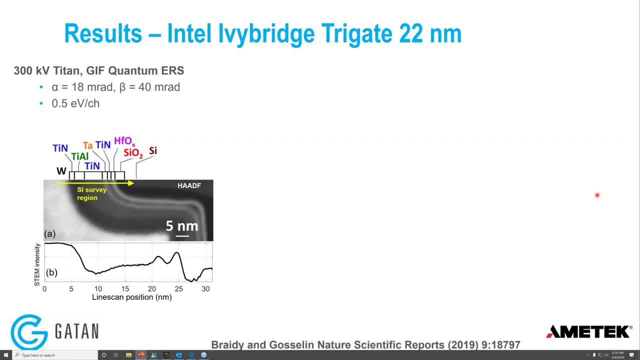 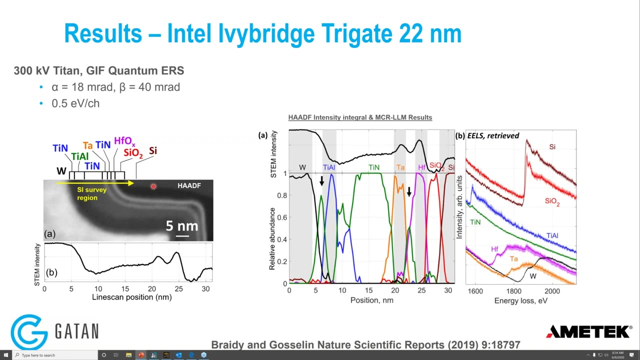 milliradians and they were running at 0.5 EV per channel dispersion. so this is the survey image and you can see they basically acquired a line profile. so the survey image region is denoted by the this yellow line. okay, so here we have the MCR LLM results. so at the top here we 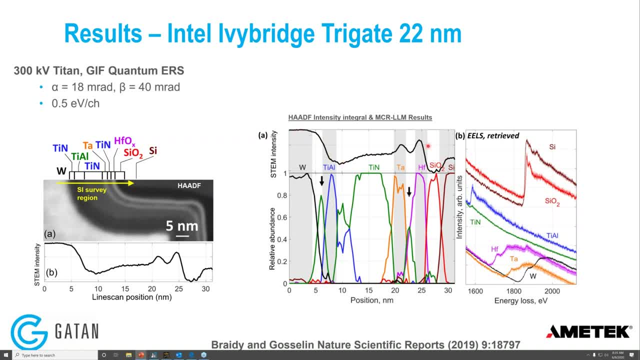 just basically have the line integral of the hadath intensity. so this is actually experimental data, the black line here, but these plots here. so this one and this one is the data that's come out of the code, so the codes pulled out these and this one is the data that's come out of the code, so the codes pulled out these and 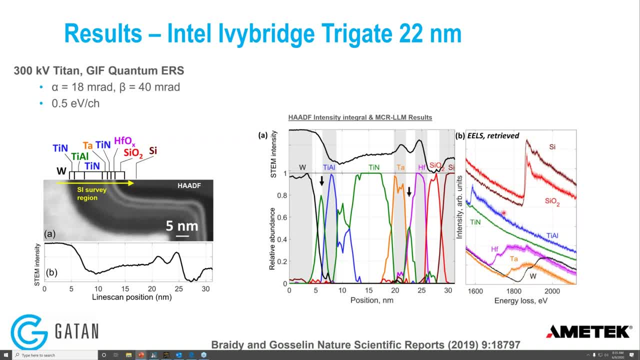 different spectral components, so one, two, three, four, five, six, seven. so we have seven components and then the other line plot here is how those components are distributed along this line, so it's kind of like intensity profiles of these spectral components. the colors: the colors match up, okay. so 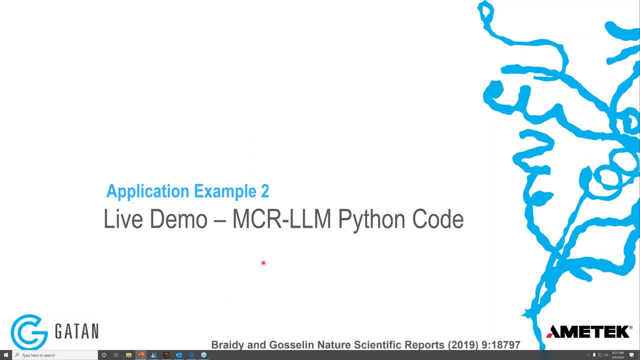 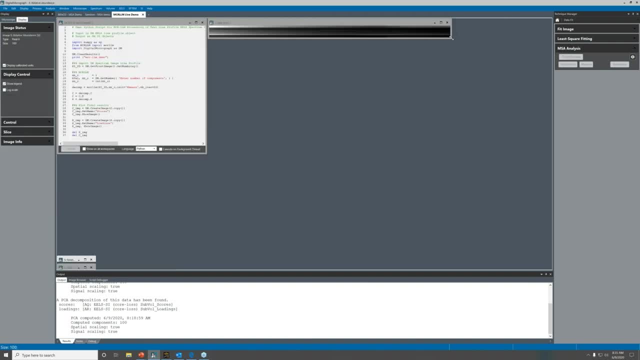 this is a good point to jump to the other demo, So MCR live demo. Okay, so you see two things that are open here. I have one that's called data eels one, So that's the line profile data. So this is the spectrum image data set. 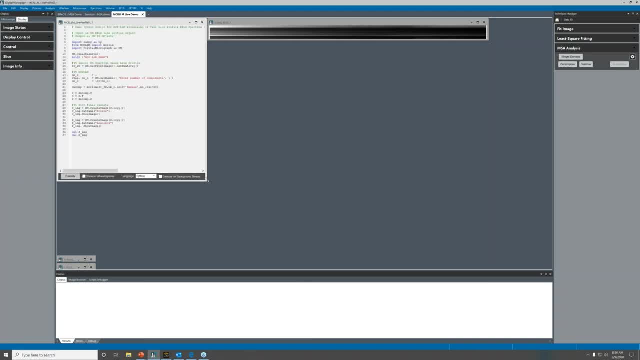 And then we have this script. So the way that the Python scripting works in GMS now is basically exactly the same as what we're used to. if anyone did Python or regular DM scripting, You just have this checkbox or kind of combo choice at the bottom where you can choose the language. 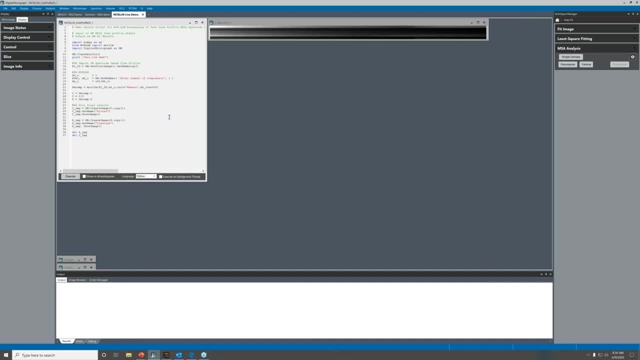 So you can choose Python. you can choose DM script, So it's Python script. I'll leave it as Python. But what's kind of obvious here? this is a really short script, So I just installed their package and this we just need to pull in the data. 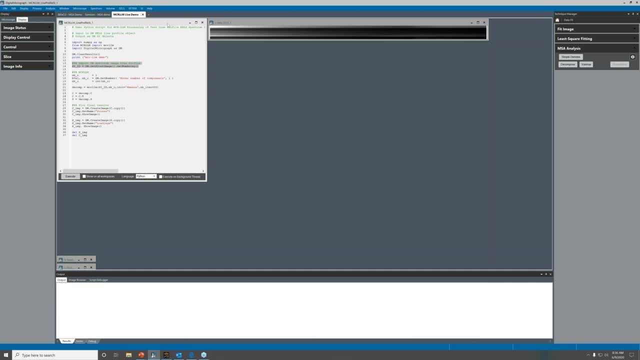 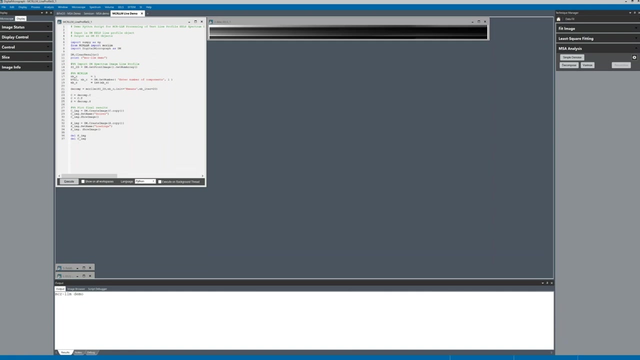 run their function and then export the data. So I'm going to execute my script. So I've added a line that asks how many components, But it's seven because there's seven components. Wait a little while, Okay, so it's just done. 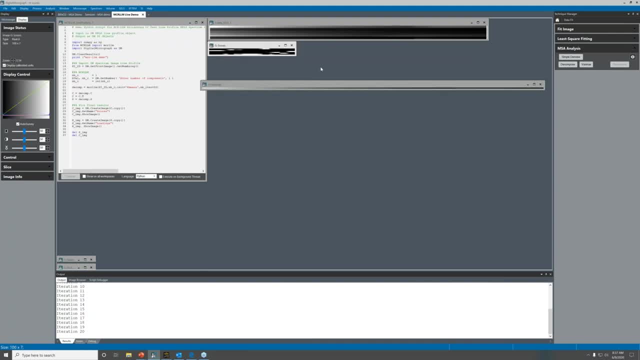 So it's just done. MCR LLM on this data set And pulled out seven components and 20 iterations. So I haven't written any code in here to convert this to EELS data, So I'm just going to do that manually because it's easier. 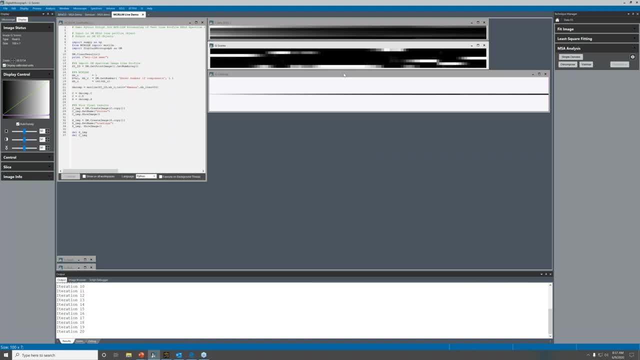 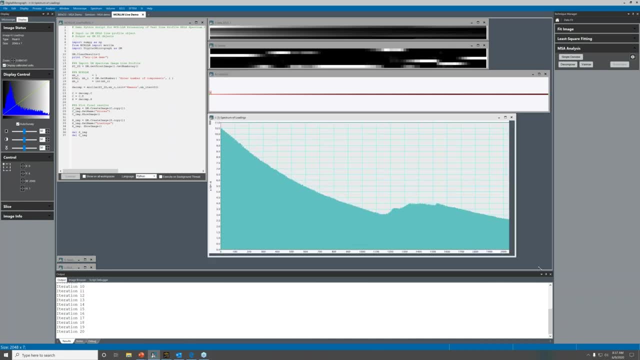 Spectrum, convert data to EELS, just for display. So that allows me to use the picker tool. So now, if I use the picker tool on this, pick a tool on this guy, So we can do so. these are the loadings, So the different spectral signatures. 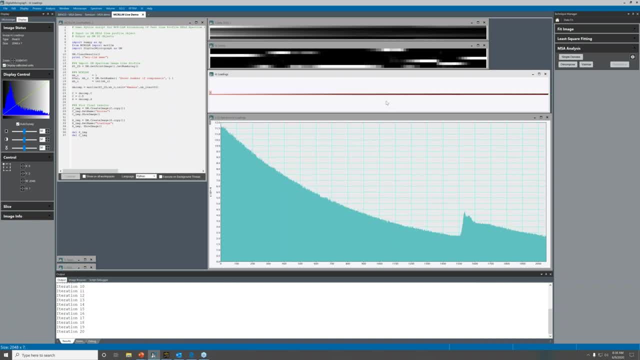 that we have. in that data There are seven- well, it was seven because I chose seven- And then this isn't actually EELS data. So what I've done here is a little obscure, but it just allows me to use the picker tool. 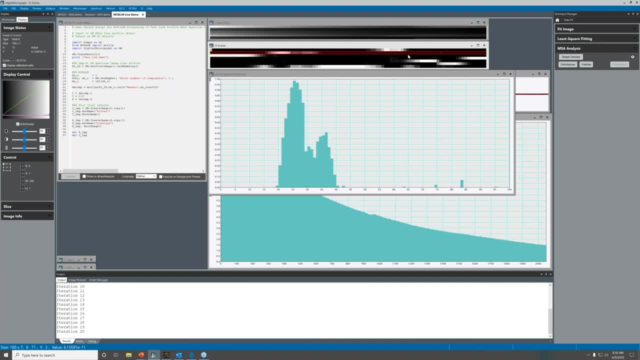 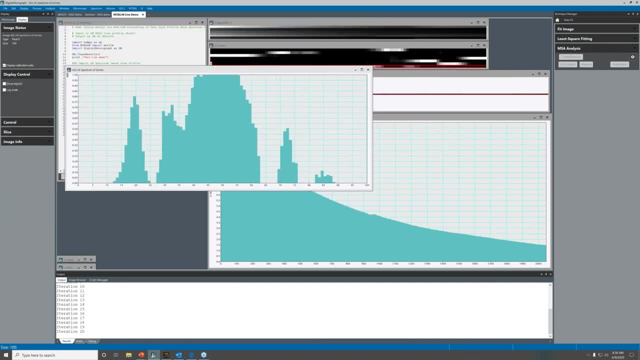 which is an easy way to kind of look at the lines. So I'm just going to do it anyway. So the score, so the scores is, yeah, just kind of how much of what we have and where. So the index is here. 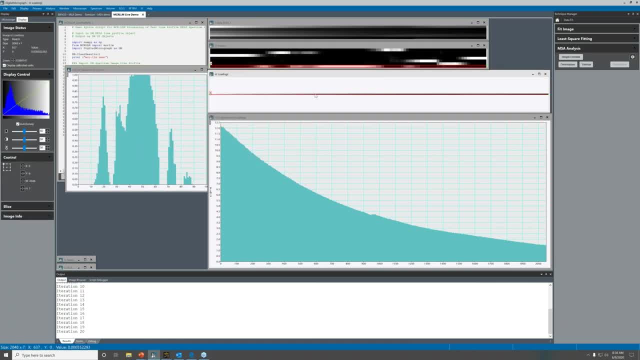 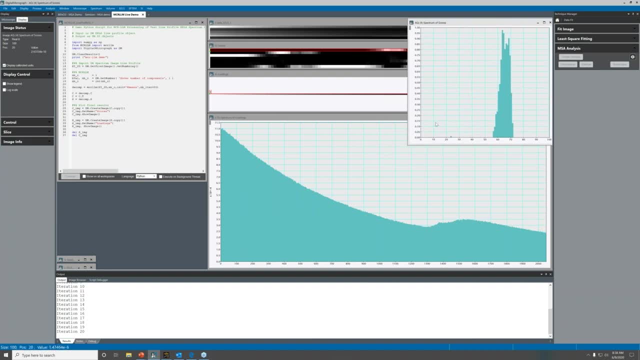 the indices match up. So this is component zero And this is component zero. So you can see that runs really fast. It's really easy. I didn't have to leave GMS to do that. And then if we look at the scripts, it's not. 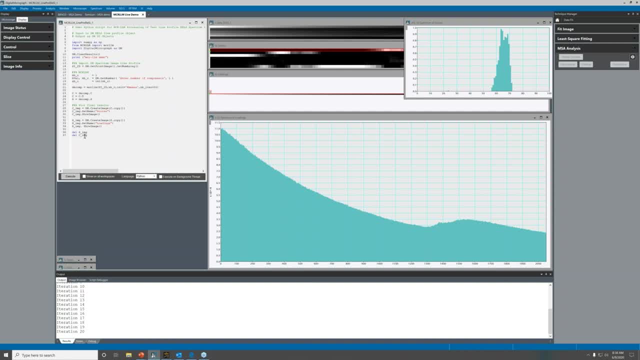 complicated script so it doesn't have, you know, 37 lines of code, including quite a lot of line breaks and comments. we could do stuff that's more fancy, like move the metadata and various things like that, but to do something that's just some easy processing, you don't have to write a whole lot of of code, so let's. 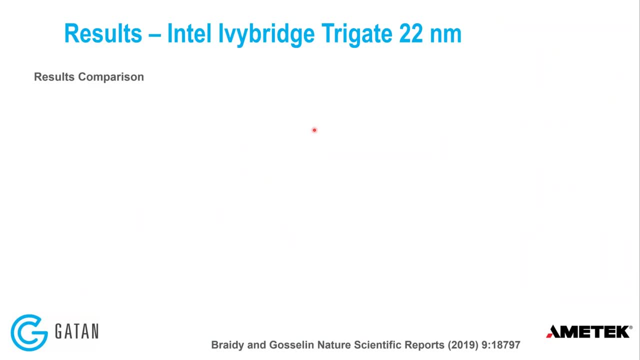 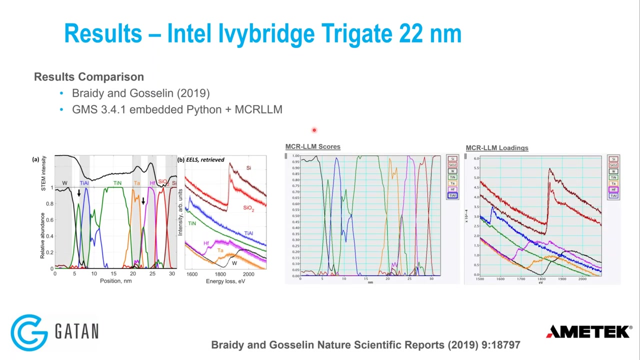 go back to the demo. so, yeah, I'll just now, yeah, compare the results. so here's the results from their paper, which we saw on the previous slide. so, and then I presented the GMS kind of output in the same way as as the results in the paper. 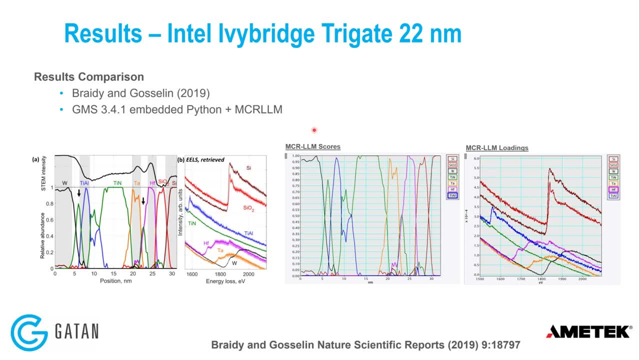 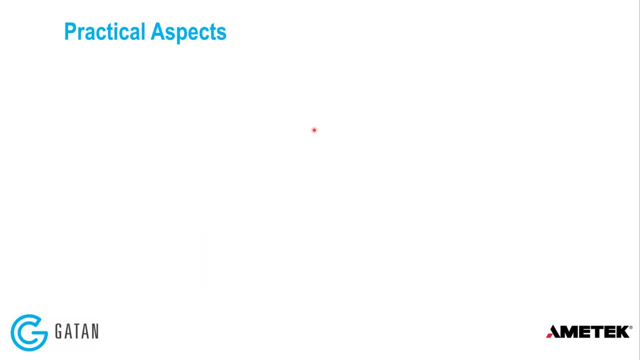 so I've matched the colors up and so you can kind of, you know, look at the two and see that they're the same. so, yeah, it's pretty nice, some practical aspects if we want to do this kind of this kind of thing. so the workflow is pretty much. you need to install the Python packages, so you'll. 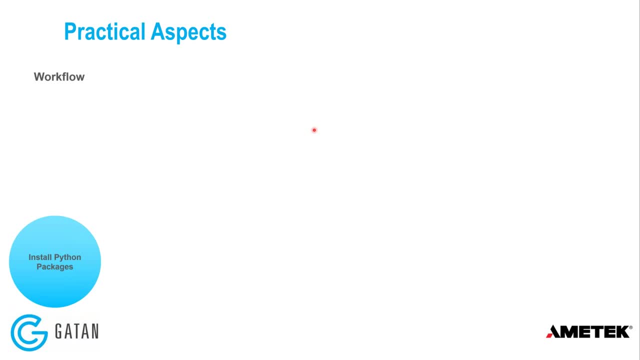 you'll probably want to work with one particular Python package, so you need to install that package and any of the prerequisites of that package needs. so maybe you might need matplotlib or numpy or or whatever. so then the first thing that we always do is convert the spectrum image data to a numpy array. that's just a single line of code. 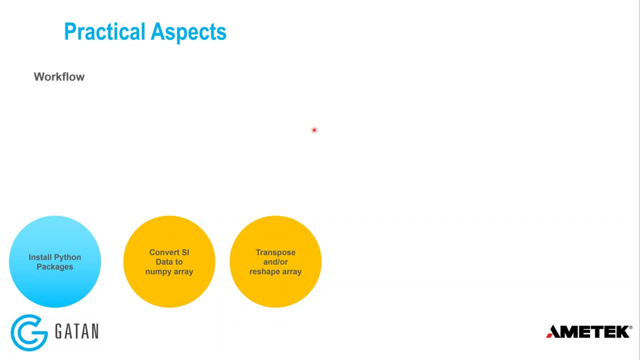 transpose and or reshape the array, perform the multivariate analysis, transpose and or reshape the output and then visualize the results in GMS. so there's really not that many steps and the bulk of this is kind of reusing the reusable for different code packages. so I've used, I've done this with a few. 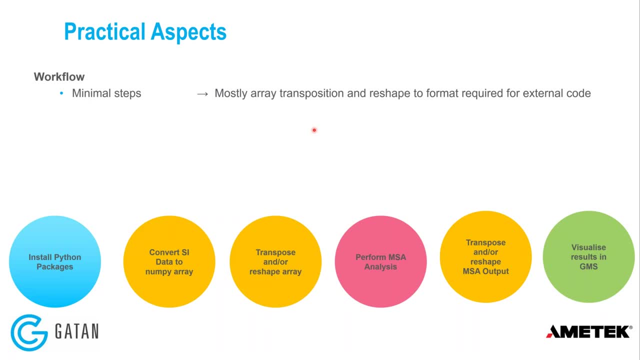 different external packages and the steps are pretty much the same. the main bulk of the work I found is to: you just need to take care with the array transpose trap. you need to be careful with the array transposition and reshape because the external code, so the external MSA code, is going to want the 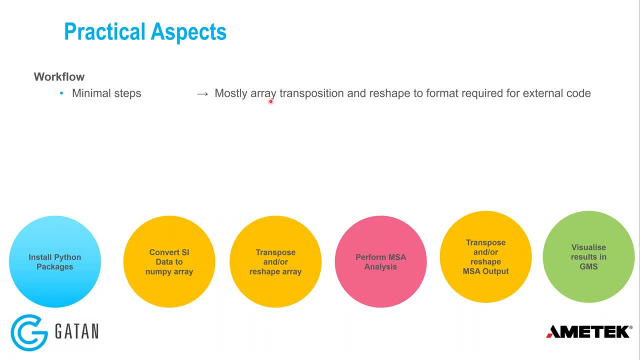 data in a certain shape and orientation, so you have to be careful to get that right, but otherwise it's it's fairly straightforward. there's some code testing tips, so anyone that has done a lot of coding this will probably be well known. but for people that are kind of 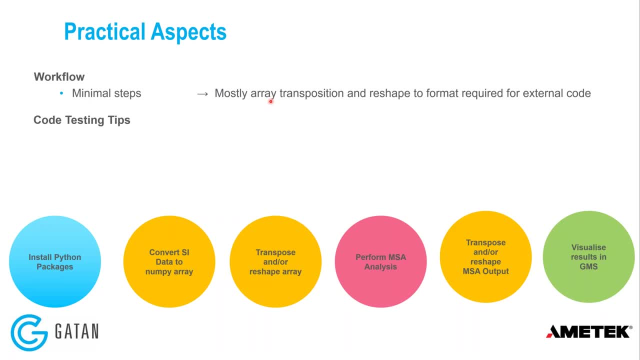 just starting out, beginners or kind of yeah, so stuff that I've picked up along the way. so read and plan. so avoid writing code before planning how the program will run. so if you basically do some planning, it will help you out a lot in the long run. 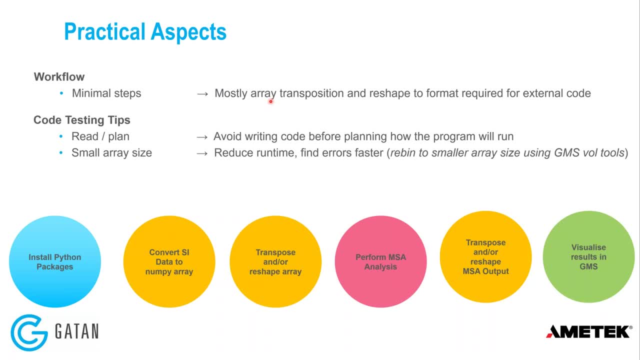 and then I just want to point out that you can do some work with small array sizes so this will reduce runtime, so you find errors faster. you can just do this by rebinding to a smaller data object size using the volume tools in GMS and then work test with asymmetric arrays. so transposition and reshaping errors are. 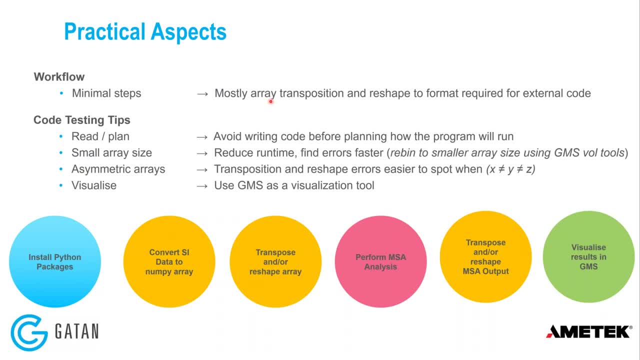 much easier to find when X doesn't equal Y doesn't equal Z and finally you have a visualization tool that you're running. so use gms as a visualization tool and just output the arrays, the numpy arrays, the dm data kind of app particular. you know you can put that test points in the code. 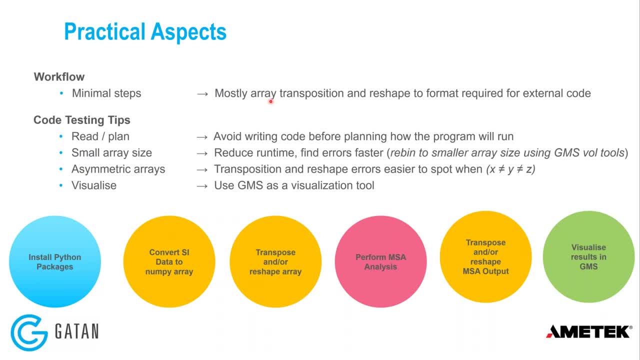 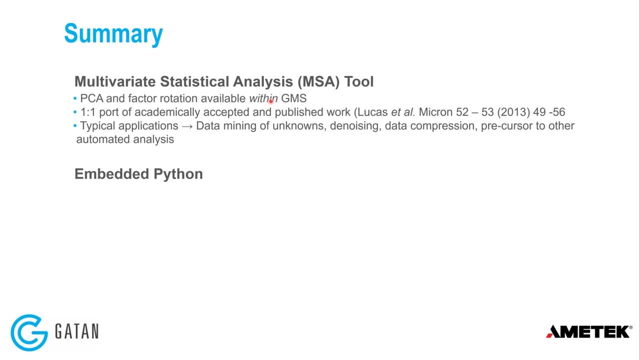 and you can just throw the array out, see what it looks like. and sometimes when you look at the array you can say, oh, it's much easier to see where it's wrong if it's wrong, okay. so summary, so multivariate statistical analysis tool so we can do pca and factor rotation within gms. 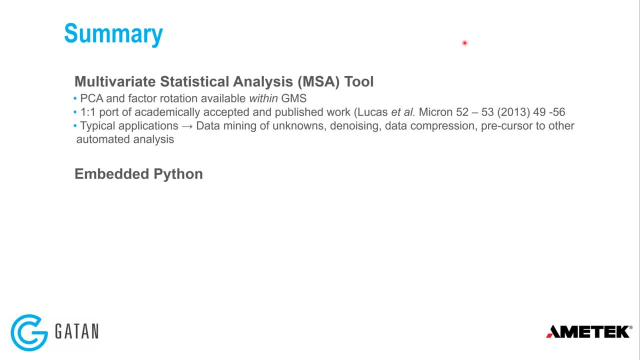 it's a one-to-one port of academically and accepted and published work, so it's published by lucas et al 2013. typical applications for the tool will be data mining of unknowns, denoising data compression, and it's a really good precursor to other automated analysis. 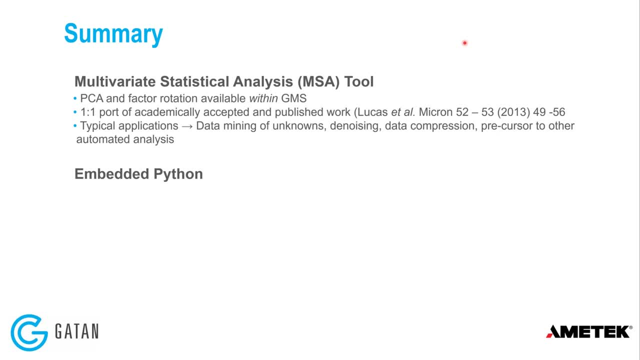 or other kind of more cumbersome multivariate analysis code. so then embedded python. so there's a lot of other msa methods that have been published and available and python really unlocks kind of access to those methods. so it's very simple and fast to install external python packages. 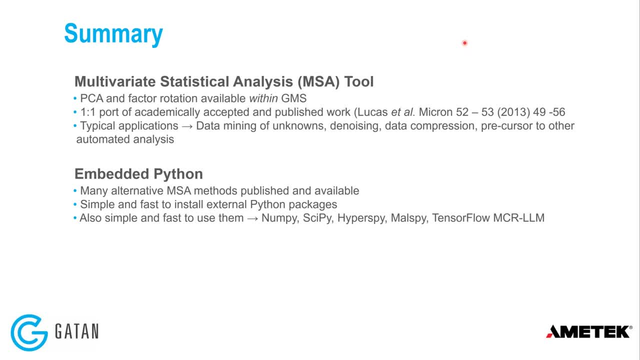 and it's also simple and fast to use them. so we have a bunch of other stuff that we can use. plus, this is all part of the free license, so you can get the software for free at katahncom and you can have the multivariate tool and the python- embedded python- a part of that free license. 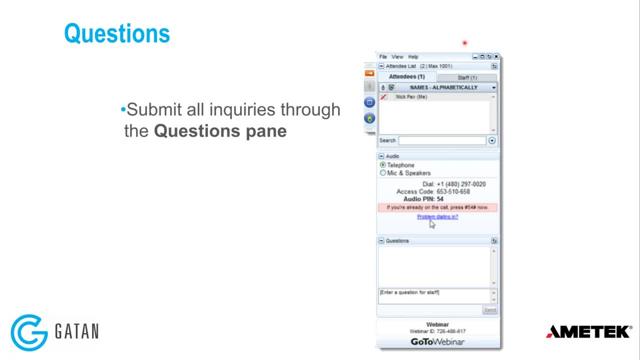 so that's, that's all. so if anyone has any questions, that would be that would be the time. great, thank you so much, liam. that was very informative. uh, those worked. examples were really nice. um, we did have, uh, some questions come in during the web page, i'm sure. what do you like? 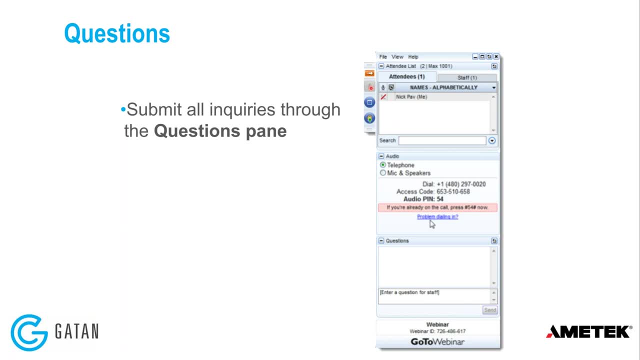 now, Leigh, that was informative. you can examine some of the questions that we've received and if you know about any of those, we can give you some feedback based on that or on our website and our specific customers, that we might partner with webinar. actually, one of them I can address straight away your question. 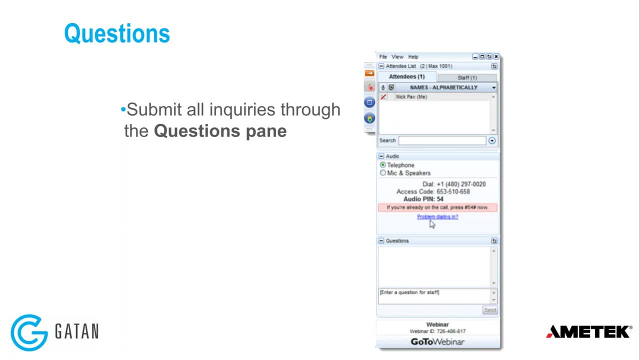 about licensing. so yeah, the free license is available on the website. if you just go to our Catan comm website, look under software in the support section. but if you already own a license for GMS 3, you can add on the functions of the free licenses together with your paid license, so the two can be combined together. 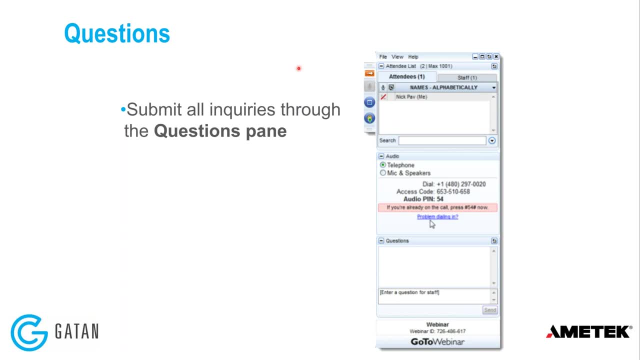 without install a deinstalling one or reinstalling the other. so if you have, say, licenses for tomography, you can then add in spectrum imaging through the free licenses and keep all, keep all of you, all the things together. so we did a question about the MCR, which I was kind of curious as well. how did you know? 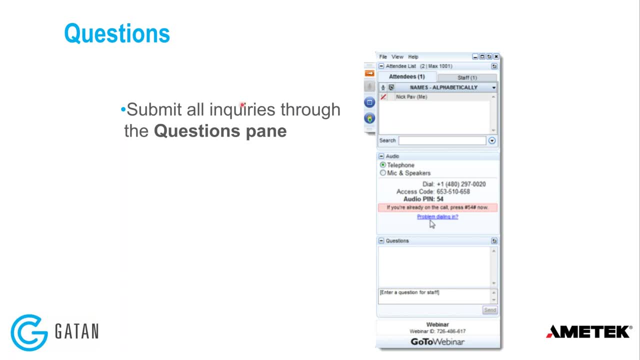 there were seven components. I mean, you read the paper, but was there a way to get at that information with you without just doing trial and error? yeah, I didn't do, I didn't do, didn't do that, but the if I probably didn't know in advance that there were seven components. 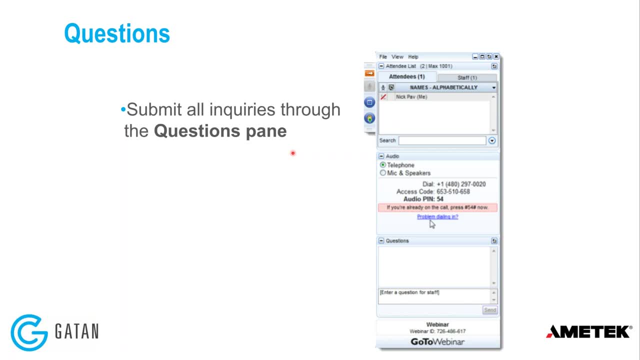 that would be a very good example of where to use the MSA tool so you could throw that data into the MSA to look at the scores, look at the loadings and look at the screen plot. otherwise you'd need to use the pick a tool on the. on the. 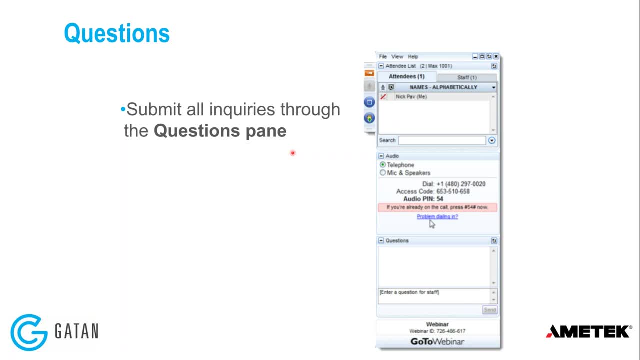 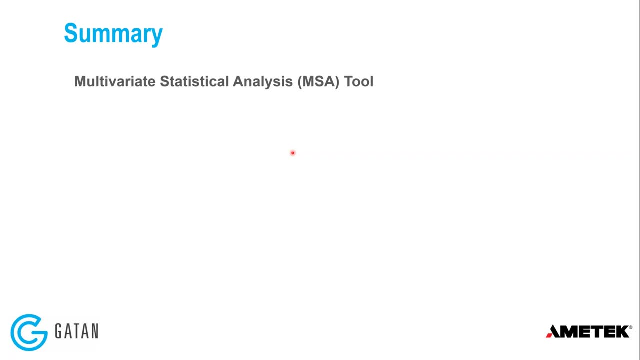 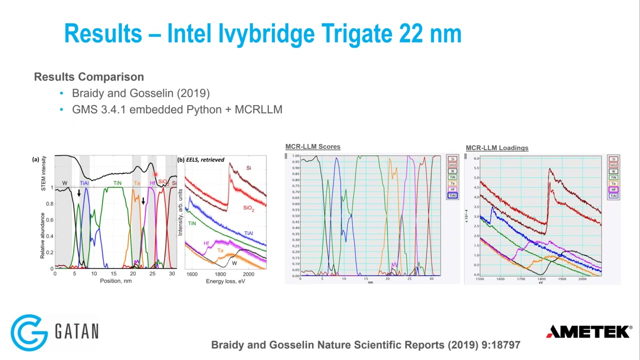 original data set for the MSA tool would be a faster way of kind of looking at the data. my opinion, especially one of those components, is very small. so I think if you just looked at the raw data it would be easy to see. it be easy to see the silicon, the silicon oxide, the hafnir, the 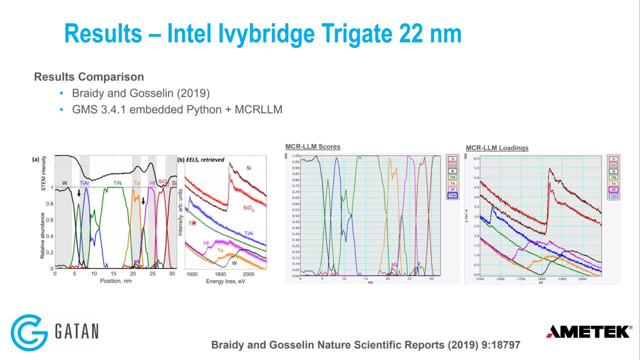 tantalum and the tungsten and the tongue. but you might miss this nitrite, this one, because that's that little bump. there is quite small, so you might. unless you looked carefully at the raw data, you might think that there were six components, not seven. so I would say using the MSA tool. 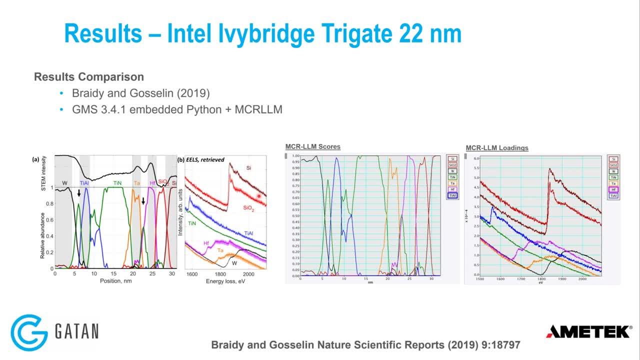 would probably be beneficial. does that answer the question? yeah, that makes sense for me. yes, yeah, PCA is good at determining the number of components. hmm, and this, this analysis was for one dimensional data, that you can also do two dimensional data. but you can also do two dimensional data. but you can also do. 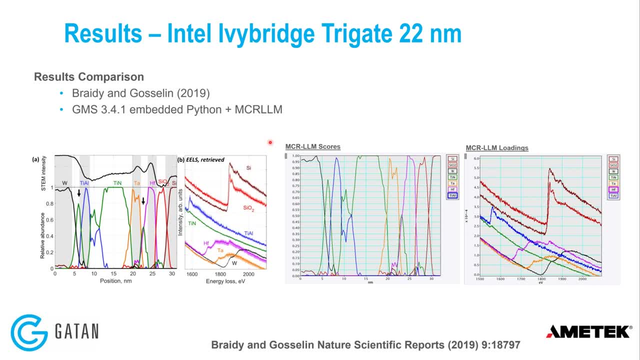 three dimensional data using. yeah, yeah, so I have two different scripts. so I have two different scripts. so I have one script that works on line profile data and another script that works on two dimensional arrays. so a 3d- 3d data cube instead of a 2d object. so I just chose to present the the line profile. 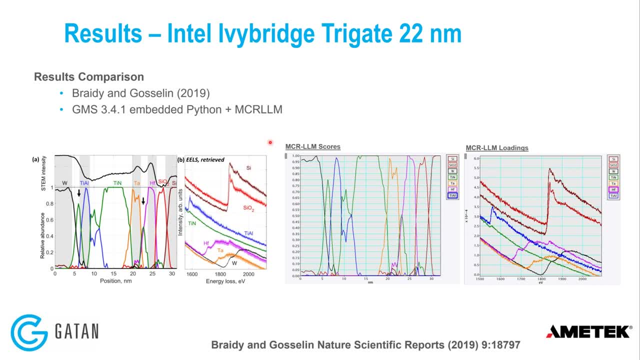 data because it was nice to compare the the work of the paper with with kind of you know what we can do in the software because we have a ary inch of of data is not cherries, zero can in. we want to see that the results are the same, but it's not limited to line profile data. you 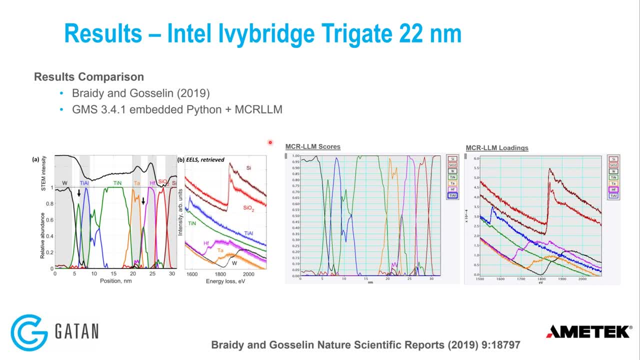 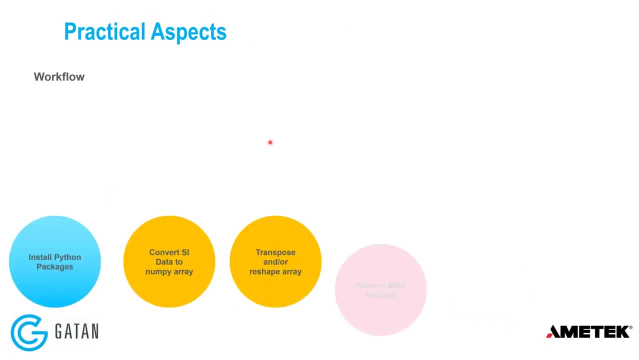 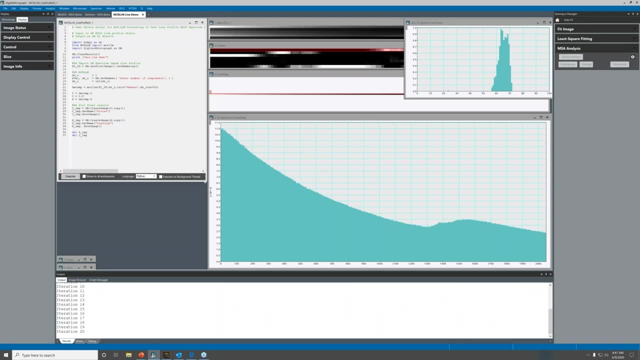 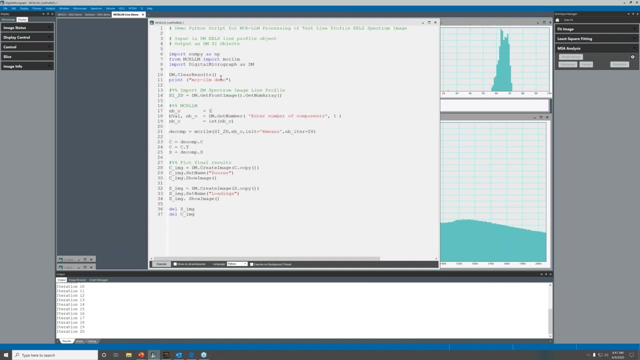 can use it on higher dimensional data. so then you just have to unwrap it differently. yeah, pretty much. so the the. where's the script? oh, it's in the software, isn't it? so it's just this step here. so you've got um, can you, is that font big enough? what is now for sure? yeah, so you've got this step. 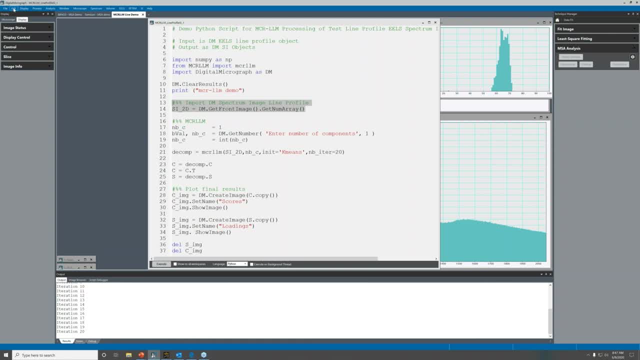 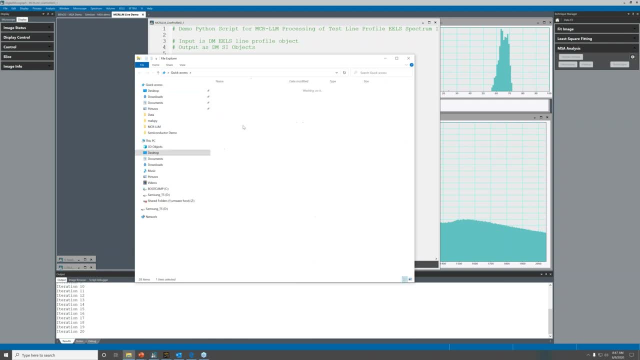 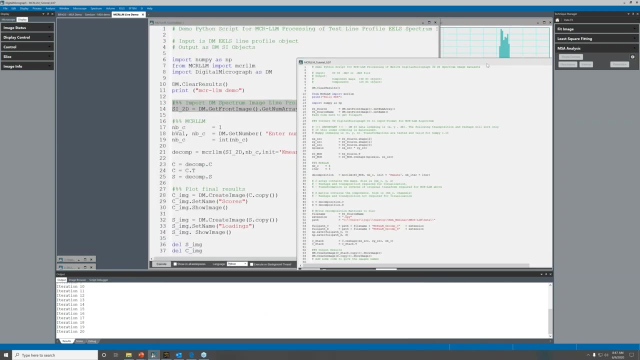 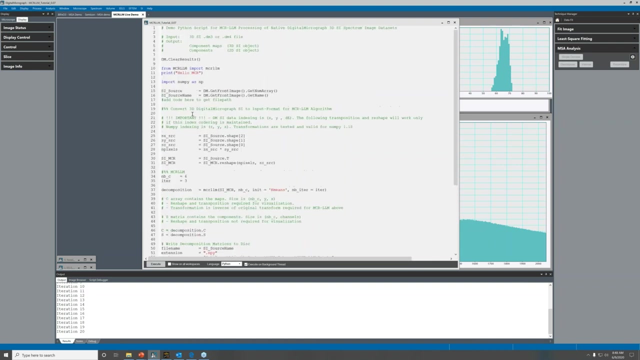 actually the line profile data doesn't really need any, any war. let's see if I've got it seven. so if anyone wants to see this code. so the line profile is in the right shape by it's intrinsically the right shape, whereas the 3d, so the 3d object- requires it. just I mean. 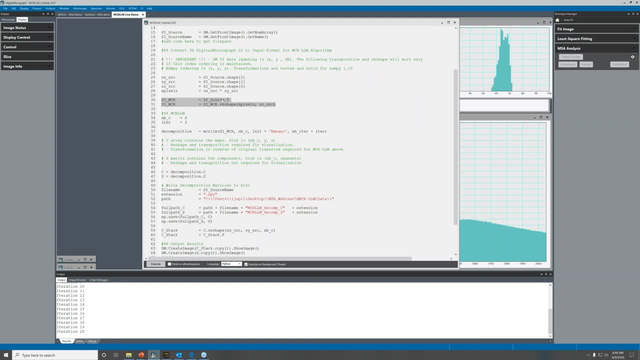 it's not a lot of code, it requires just so. the way this code works is it takes line profile data. so what you have to do with a 3d object, you basically you have to do a transposition and then you reshape the transposed array into. 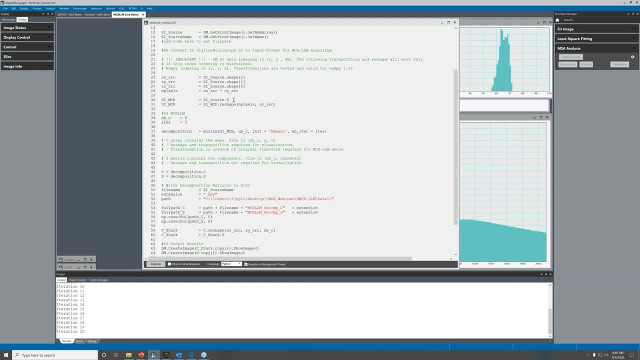 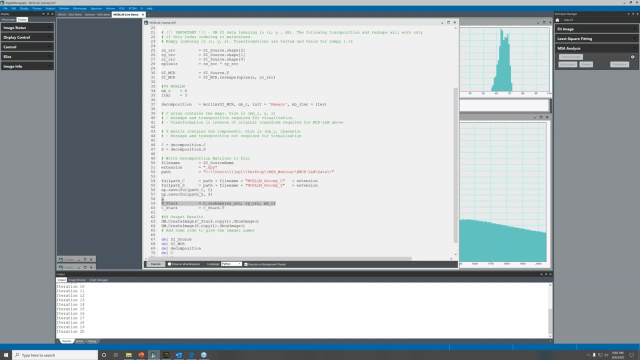 a line profile, so it just makes a much, much bigger line profile for the input, for this mcr code, and then at the end then you have to reshape the, the result into something. so it's just essentially three lines of code. you do this transposition here, reshape, and then the mcr. 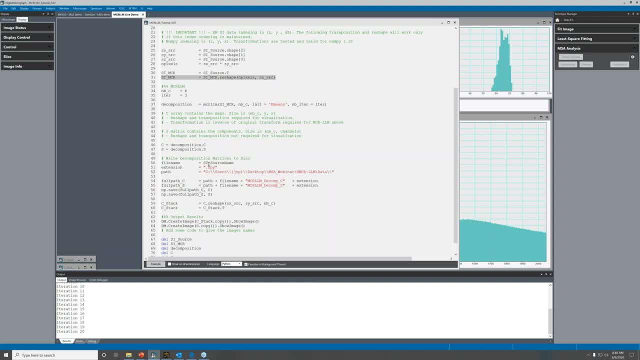 does its stuff. I mean, a lot of the code here is just safe. I actually have some extra stuff here to save the numpy array to an external file, but the actual mcr part is really just this line here, so there's a single function. yeah, so it's this function. right, you've got. 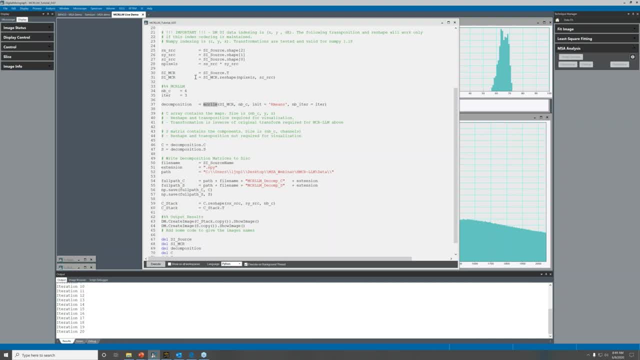 a function called mcr llm that you call on an array and you've got some parameters, so number of iterations or number of components. yeah, basically it's an array, a number of components, a number of iterations, and that's what you're going to do with the 3d object. so you've got a 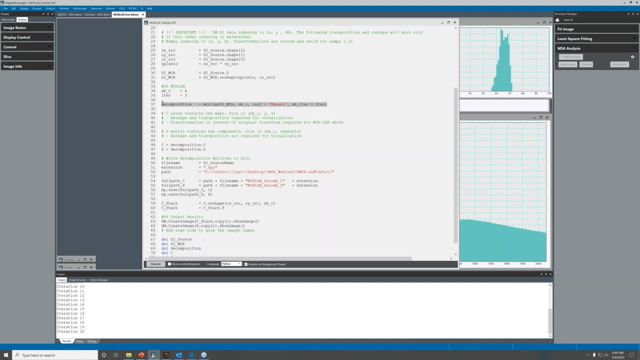 it. so you just have to put something into this. that's the right shape. then you get your C and S matrices out and then you reshape the C matrix so that it looks correct in digital micrograph, but you don't need to do anything with the S. 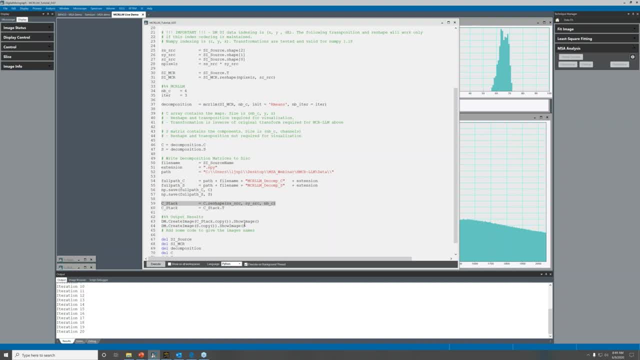 matrix. the S matrix is the right shape, so it's just. that's really the main thing that you have to do. it's just getting getting the data in the right form for the whatever code you want to use, and just don't assume that it will be the same. you do it once it. the steps are the same, but the actual the 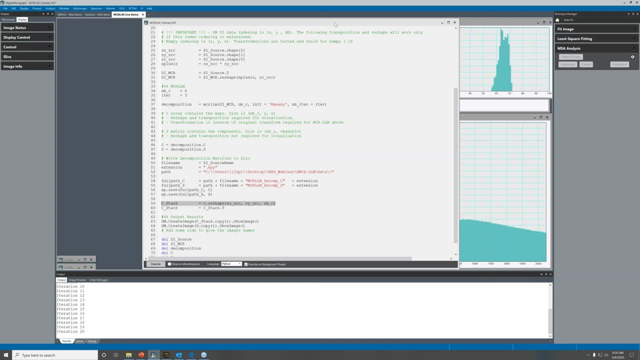 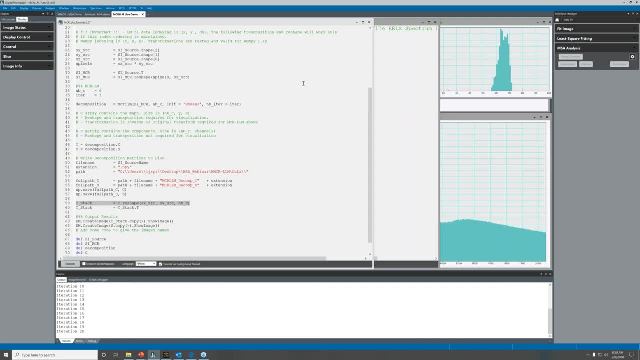 implementation is usually slightly different, so it's worth. it's worth just checking, checking that, and it saves you a lot of time. yeah, I don't know, I've gone off on a bit of a tangent, okay, yeah, I guess I kind of sent you off there, so 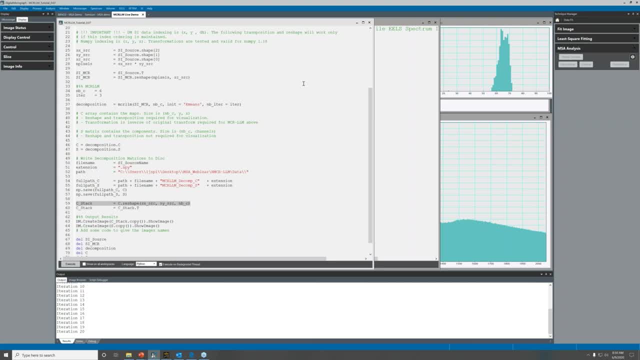 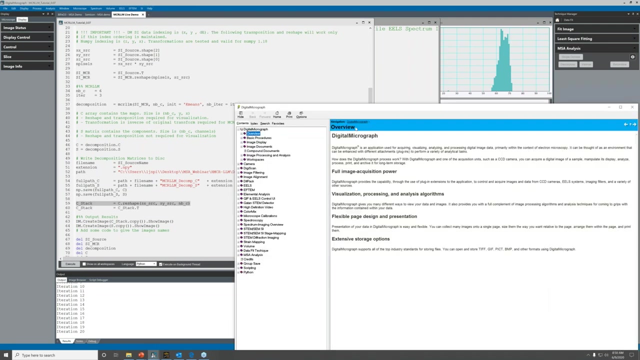 actually a question from from me is the, the, the. so I'm kind of new to the Python scripting, the. there's a in our help file. we have examples of Python scripting and different ideas like this. I think there is one version with the using a negative, non-negative matrix factorization that. 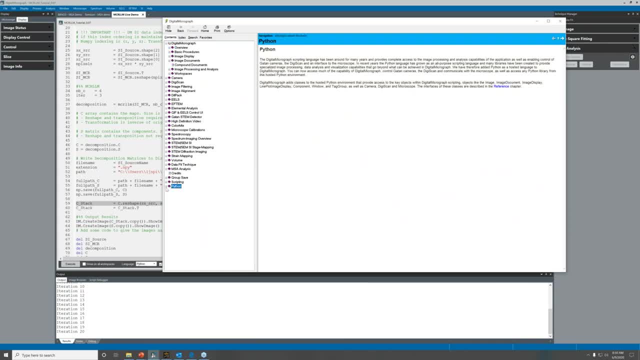 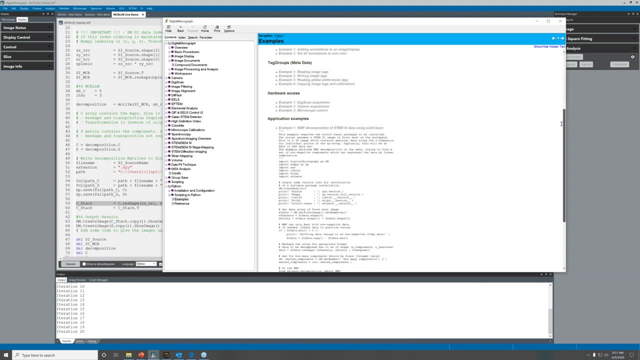 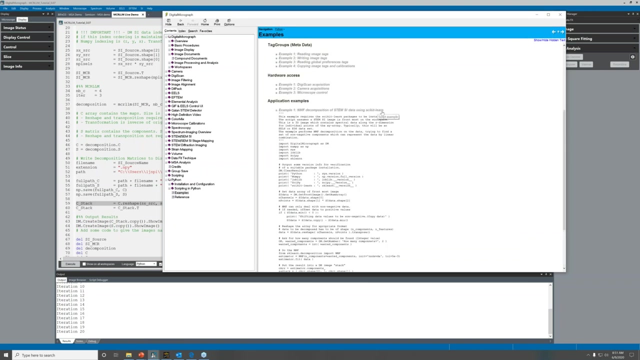 is correct. so there's a Python scripting um section and if you look in the examples, one of them is NMF. so you've got that. I'm not sure I can zoom in to that very much or at all. yeah, exactly, so there's an. there's an NMF example here using the psychic. 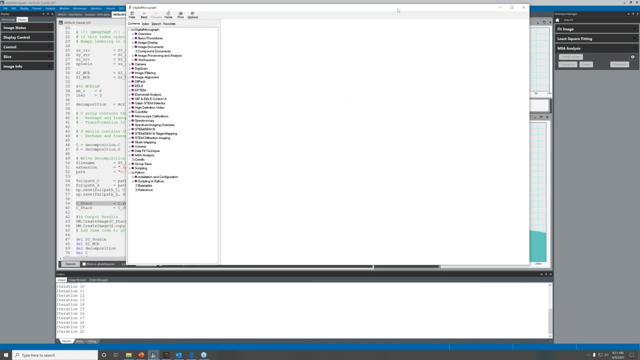 learn package, so you just need to it's. so yeah, you need to install sklan and scipy so that this and at the NMF in scikit-learn works really nicely with EDS data. yeah, it works pretty well. I have some other package that works better with eels. that is so, if anyone is. 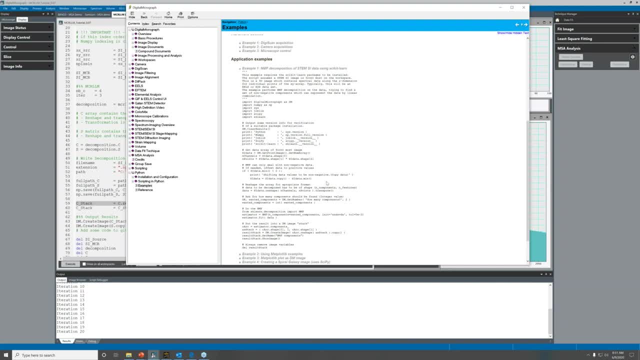 interested, just reach out. and it's a package called mouse by that seems to give nice results and it was published by a Shiga group and, yeah, you know, in Japan I think their code has some more kind of exotic sort of constraints that you can put on the NMF that seem to work better for eels and just the standard. 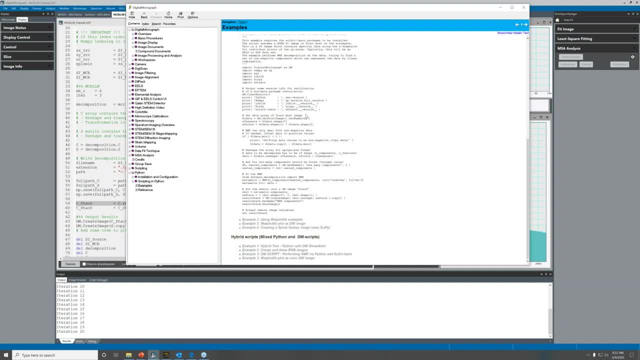 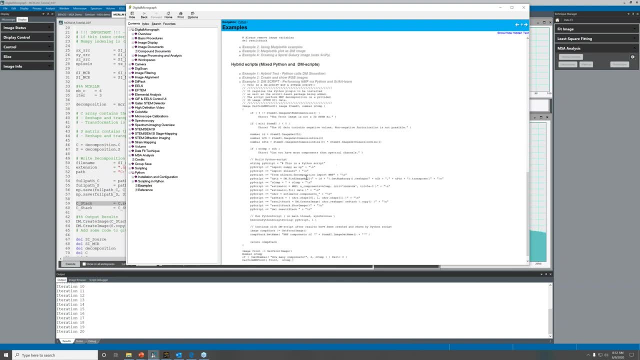 algorithm. but yeah, this is a nice example and there's also an example like a hybrid script, so you can- actually you can- embed the Python code in the DM script code, so that's kind of cool, so you can call the Python script from within the DM script, which is so that example, if anyone's interested in it's. 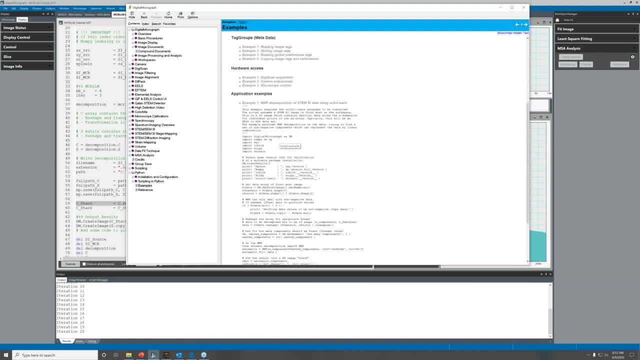 probably worth working on this one. first, just the NMF decomposition, and then look at the. the second one, which is a hybrid of DM script and Python script, wherever I just put that somewhere in there. that one example, three, yeah, okay, great, yeah, cool, and I think that's it for this presentation. I know we have a couple. 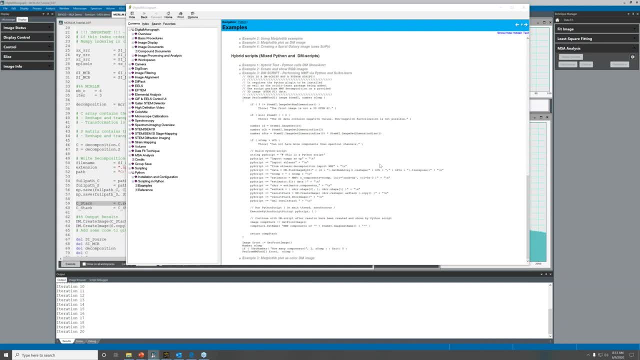 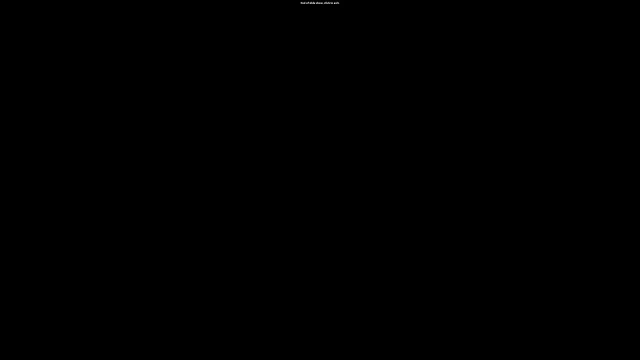 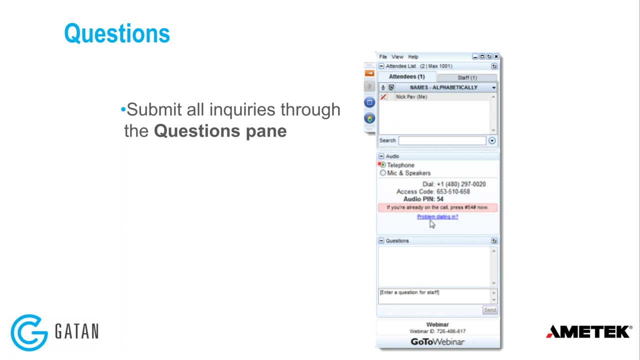 minutes over already, so maybe we should just leave it there. I do just take a moment just to thank you, Liam, for the great presentation, thanks to the group at EPFL, Susanne Libera and her team there for sharing the, the code base for the PCA, and Natty Brady and his group there at Sherbrooke for helping us out with. 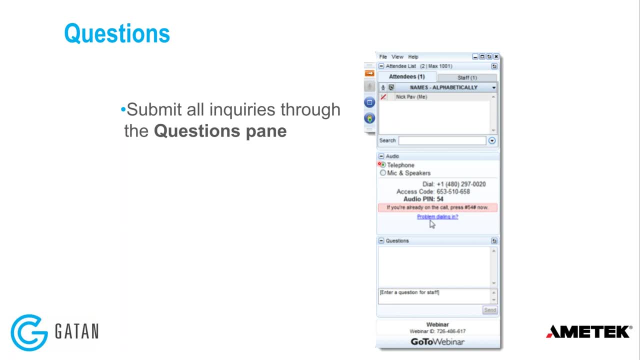 the multivariate curve resolution, And I guess the next webinar is not in the same series but it's on 23rd of June and it'll be the group at the Center for Integrated Nanotechnologies at Los Alamos Lab and Sandia. 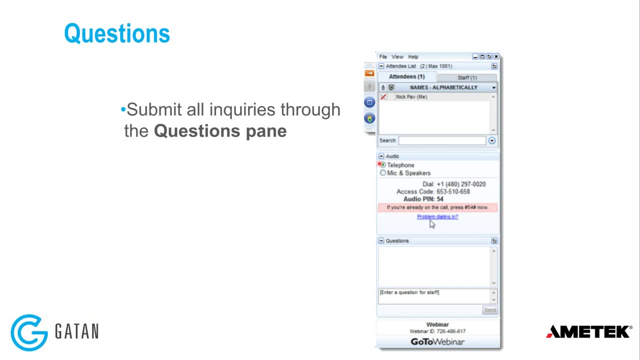 Labs, talking about institute analysis and high-speed data, so that should be very exciting. So again, I want to thank everybody for joining and tuning in. If you have any questions, keep them coming. We'll try to get to those questions offline and appreciate your attendance. 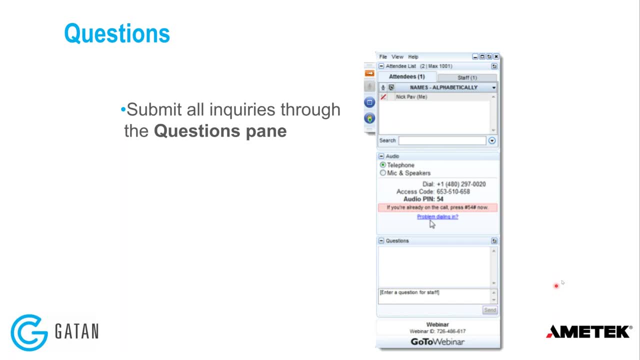 Thank you very much, Yep. Thanks everyone. Thanks, Ray, Awesome.